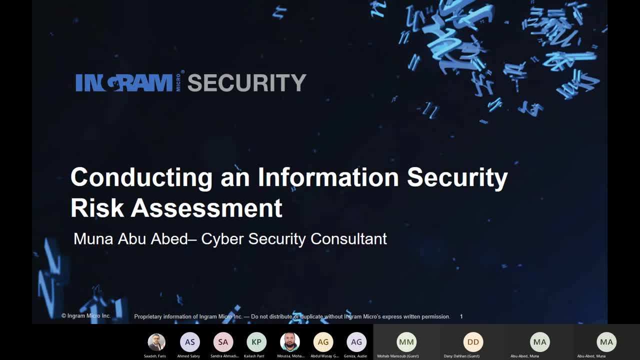 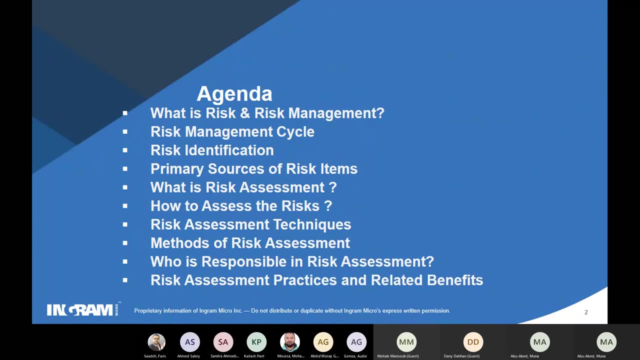 is the risk assessment, the risk identification, and how we conduct an information security risk assessment. So in my webinar today, I will speak about what is risk and what is the risk management, and then what is the risk management cycle, the risk management identification. 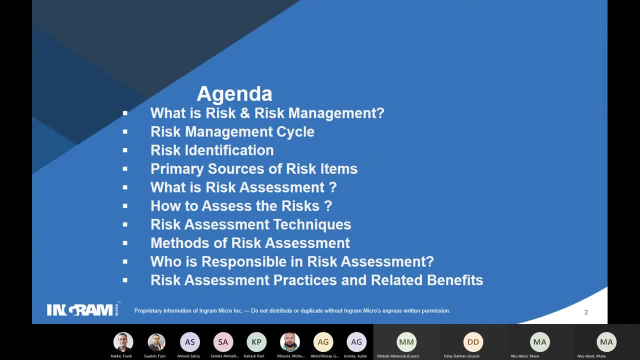 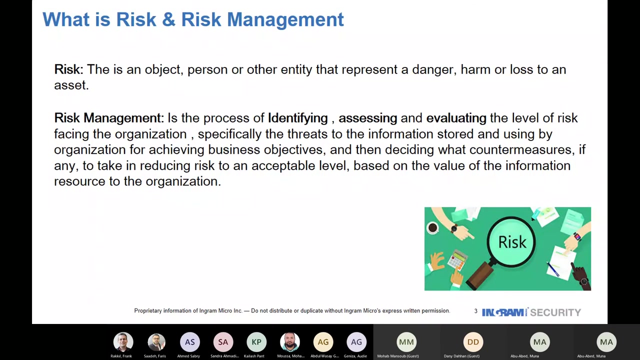 primary sources of risk items. what is risk assessment, how to assess the risk and also risk assessment techniques, methods of risk assessment. who is responsible for risk assessment, risk assessment practices and related benefits. So first of all, let's speak about 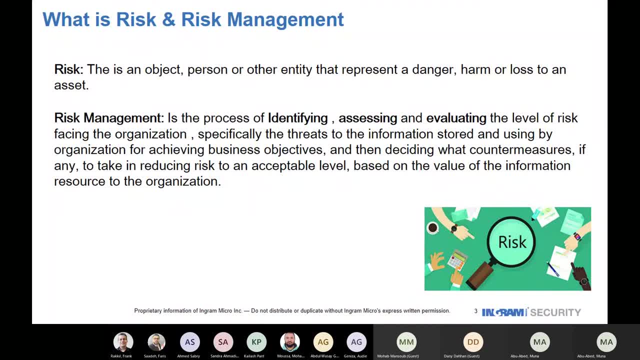 what's risk and risk management? So, as I mentioned, we all heard about something called risk in cybersecurity and I'm sure that you heard a lot about risk assessment, risk management. So we are saying risk. what we mean by risk? Mainly risk is an object or person or other entity. that 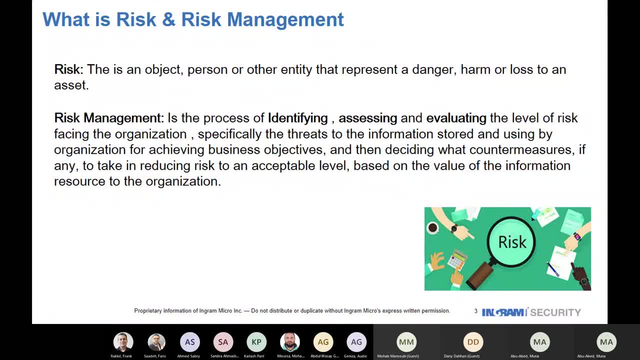 represents a danger, harm or loss to an asset. So the risk management is the process to identify actually and then assess and evaluate the level of risk that's facing the organization. So risk management is a process that takes a risk assessment to guarantee the safety. 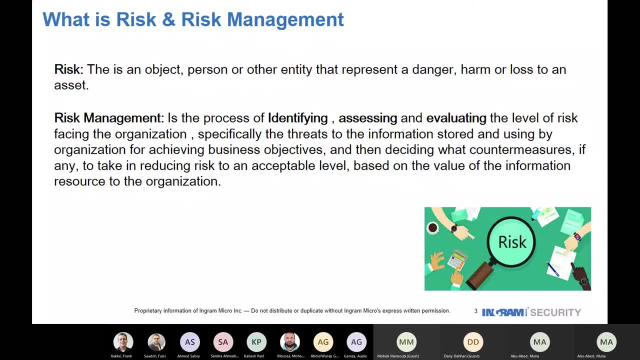 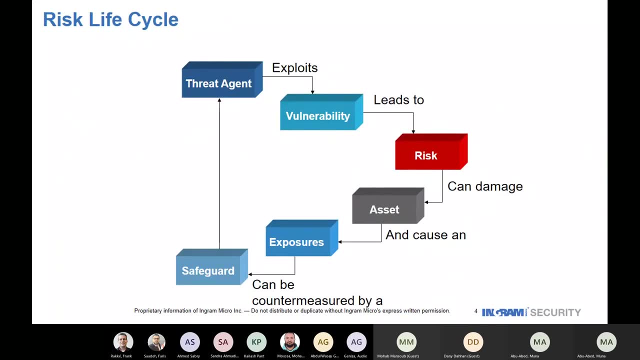 of the organization. So the risk assessment- risk assessment is the process that takes the risk assessment into account, based on the relationship between the risk assessment services and the risk assessment. So the risk assessment process is essentially- which is really very important- that threats to the information stored in the organizations. 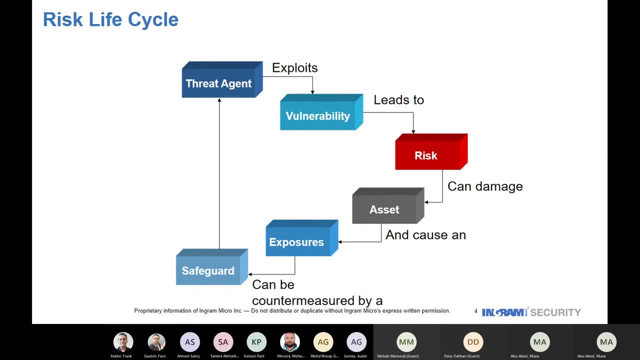 I tried to make it so simple in this paragraph, actually. So imagine that we have a risk or a threat agent that exploit a vulnerability and this will lead to a risk, And, of course, this risk can damage the assets and this will cause an exposure. 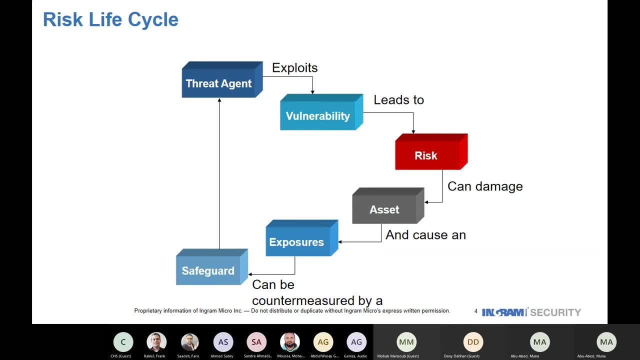 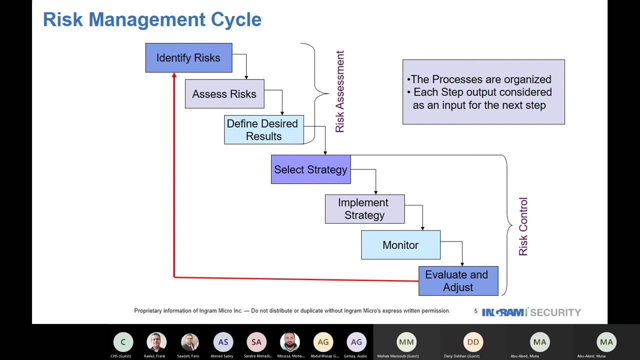 And then, after doing, let's say, the risk identification, if we pass it through this life cycle, we need to have a countermeasure and to use specific safeguards to prevent the risk or to limit the risk. So when we are saying risk management, as I mentioned, it's a process of identification, validation. 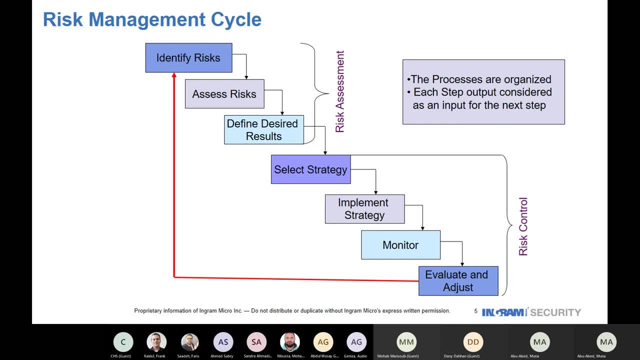 And then a safeguarding from specific risk. There is a specific risk management cycle that we used to rely on when we do the risk management, So I put it in this simple way. So there is identify the risk and then assess the risk and define the desired results. 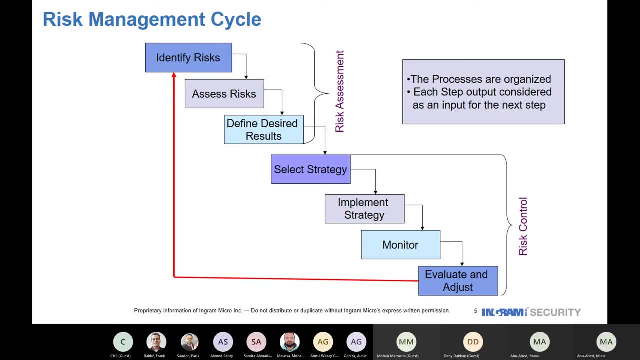 And this is under the umbrella of the risk assessment. So When we do risk assessment, of course we identify and assess the risk and based on our make it, based on some defined desired results, And then, after we do the risk assessment, we do risk control. 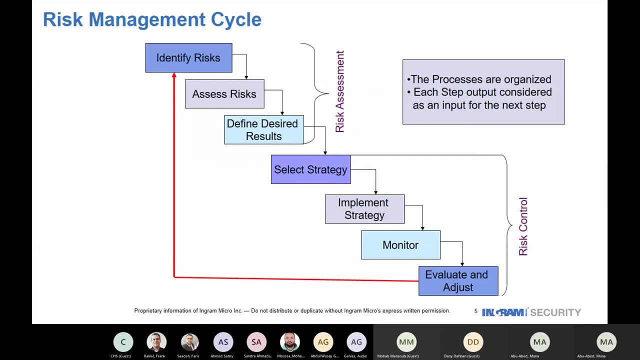 So we select the strategy, because there is lots of risk management strategies- and then we implement the strategy, we monitor and then we evaluate And adjust the risk, And this is something we deal with it as a loop, So we don't stop on evaluating and adjust the risk. 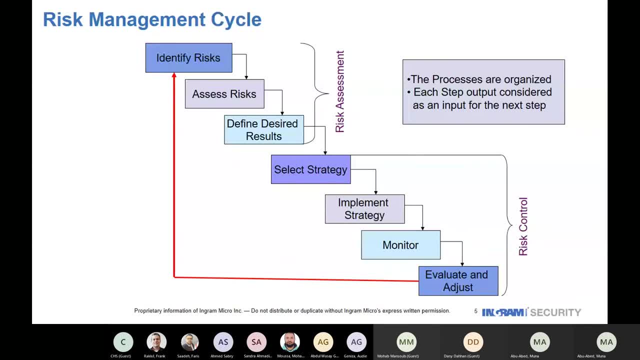 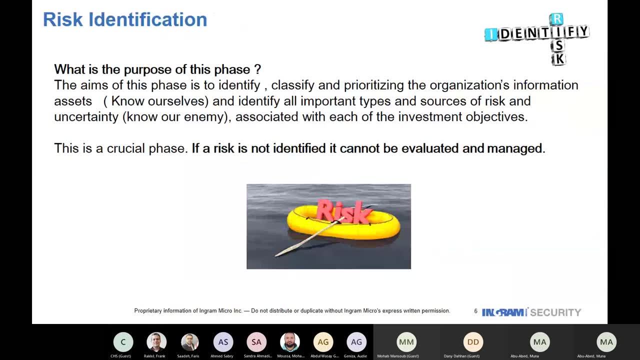 We keep identifying the risk and assessing the risk. So we go through again the risk assessment and then the risk control. So we spoke about the risk identification. So what's the basis, So what's the purpose of this? We say in the risk management, the first phase and the most important phase is the risk identification. 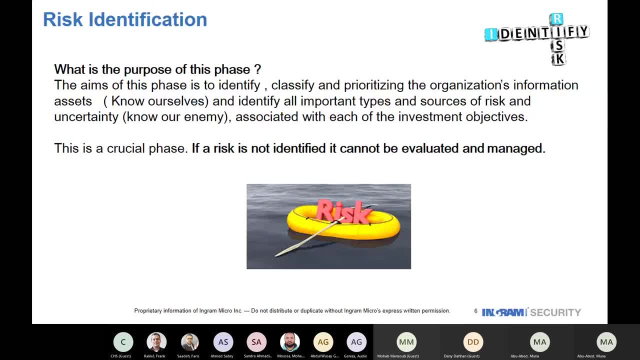 So what's the purpose of this phase? As I'm mentioning here, the aim of this phase is to identify, classify and prioritize the organization information assets. So we should know what we have, We should know ourselves and identify all types of sources of risk. 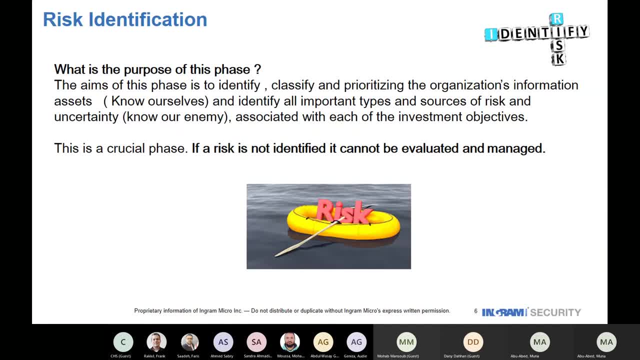 And the uncertainty- we should know our enemies as well- and associated with each of investment objectives. So, of course, when you do, it depends on the sector that we are dealing with or we are working with, or the- I mean the sector that we are doing, the risk management for it or the risk assessment. 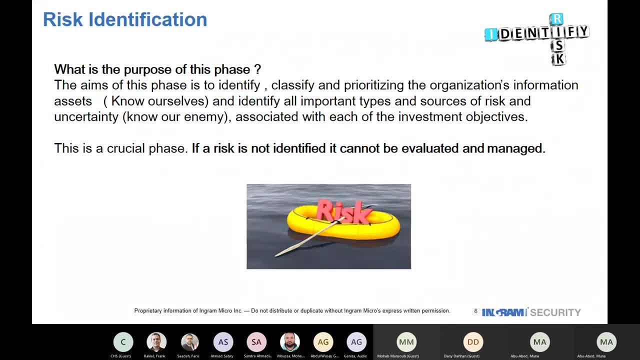 So the baseline, the most important, The most important thing, is to classify what you have to classify and prioritize your information and your assets and your resources of the risk- And it's defined from an organization to another organization, even in the same sector- depends on their objectives. 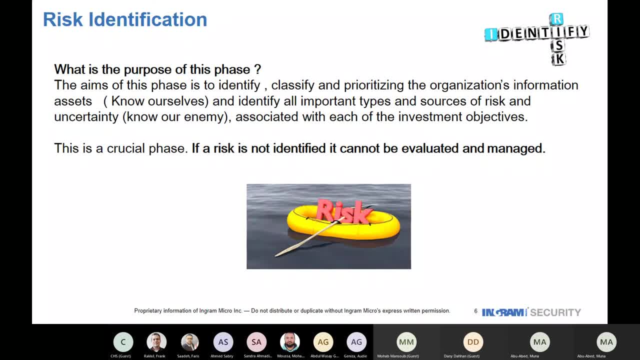 OK, so As as it's a baseline, So it's a crucial phase. If you didn't identify well the sources of the risks And If you prioritize and you classify, you identify well, And if the risk is not identified, it cannot be evaluated or managed. 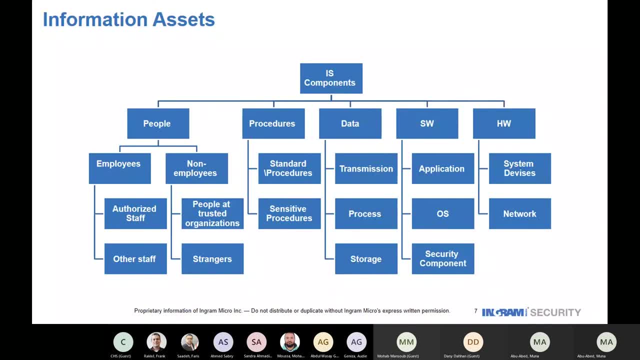 And this makes sense, right. When we say information assets, So let's look at the picture from a high or a top of you. So when we are saying information assets, what's the components? So we're talking about the people. So those people- maybe they are employees or non employees- 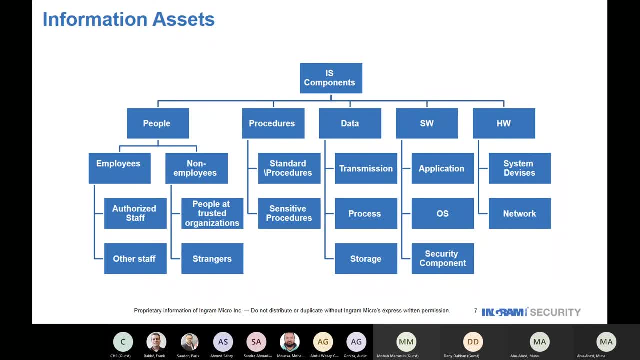 And then we need to classify the employees, to authorize the staff and other staff which might not be authorized, And the non employees, people at trusted organizations or guests or strangers. So, and the second thing is the procedures. So we have standard procedures and sensitive procedures. 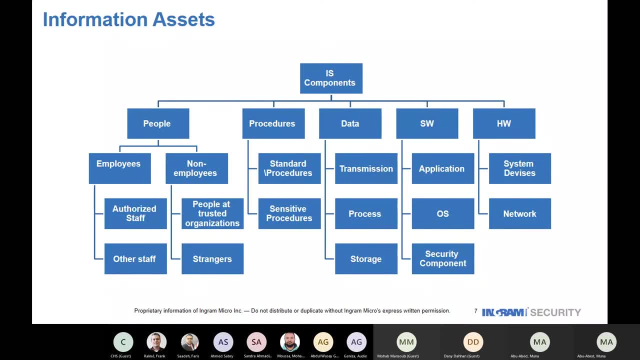 And then the data, So you need to check all kinds of data which you are storing. So data and storage, and under process and in transmission as well. And then the software and the hardware that their organization has. So under the software, you need to classify your applications, operating systems. 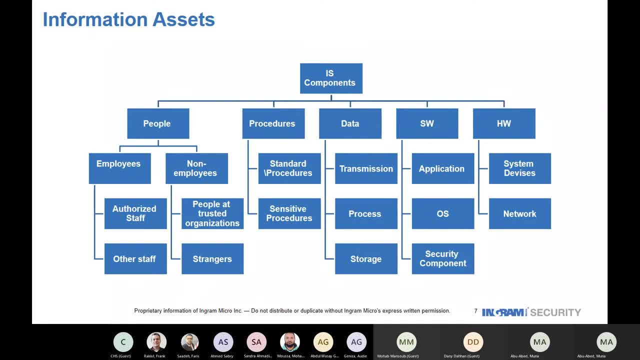 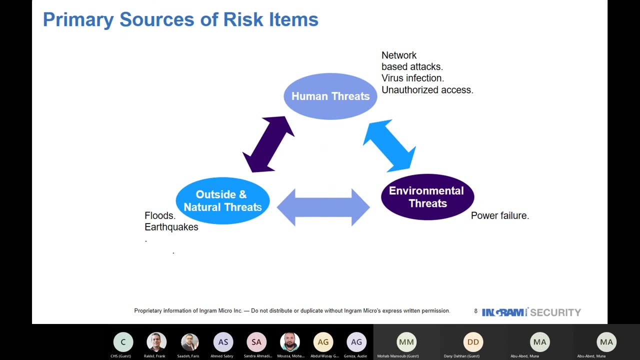 And security components And under the hardware, of course, you need to classify or identify your system devices and your network devices as well. So we spoke about the risk, the risk management and the first phase, which we said it's crucial phase, which is the risk identification. 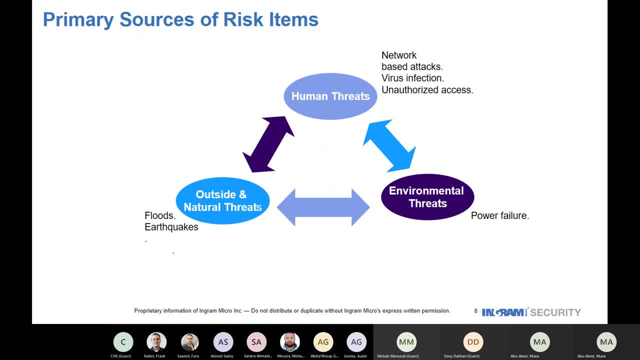 So what's the primary sources of risk items? The first source is human threats. So when we are seeing human threats, for example network based attacks, virus infections and unauthorized access, And then the second factor is the environmental threats, which is the power failures. 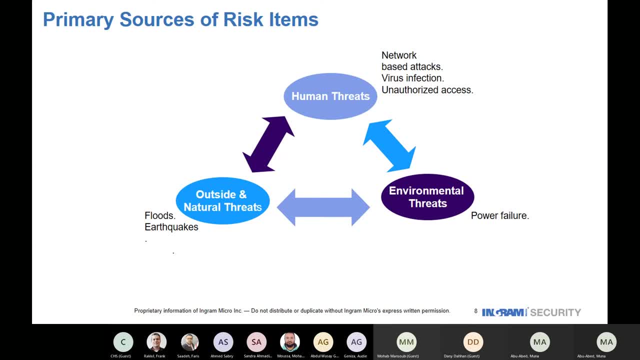 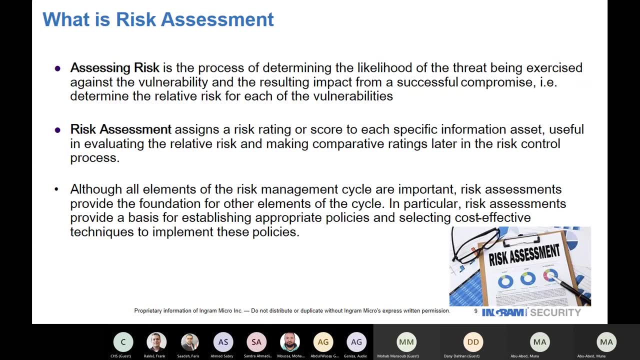 And the third one is the outside and natural threats, Such as the earthquakes and the floods. So what we are doing in the risk assessments, What's the risk assessment? So, when we are saying we need to assess the risk, we spoke about identifying the risk. 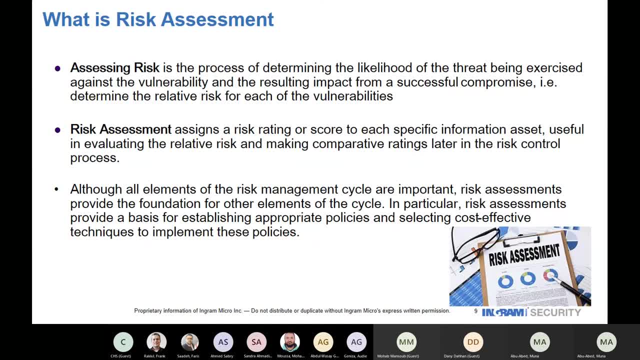 And we said it's the process of categorizing, or put the sources of the risk Under a specific category, And you need to categorize your assets, which is in the component, And we saw what is the information security components actually And how, the simplest way to classify them to be able to see the source of the risk. 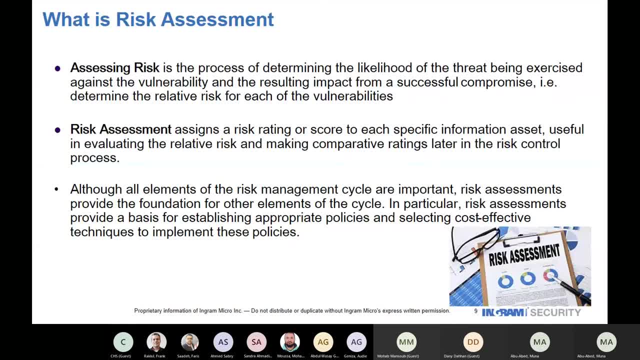 So if we pass it through all of these steps, then we need to do something called risk assessment. So what's the risk assessment? So assessing the risk is the process of determining the likelihood of the threats being exercised against the vulnerability And resulting the impact. 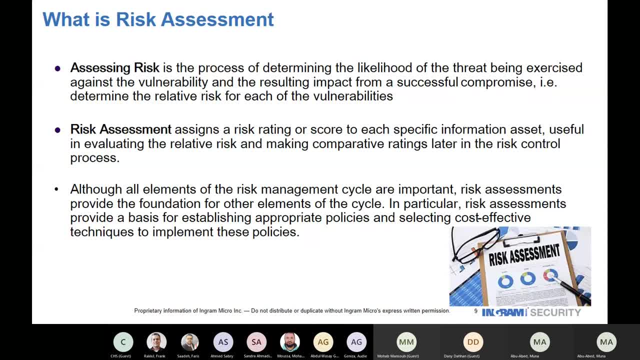 So we have likelihood of happening And we have vulnerability. And then what's the impact if this, let's say vulnerability, happened, With the likelihood high or low? So we need to actually list the likelihood, We need to list the impact of each, let's say, risk resource. 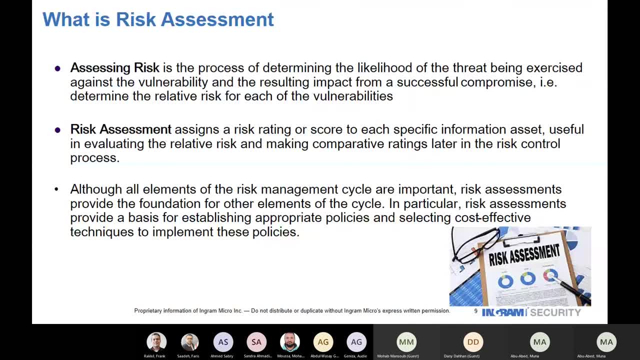 And this is how we are assessing the risk. So, for example, determine the relative risk of each of the vulnerabilities. So risk assessment assigns a risk rating to score To each specific information asset. So imagine that we have a big list of assets. 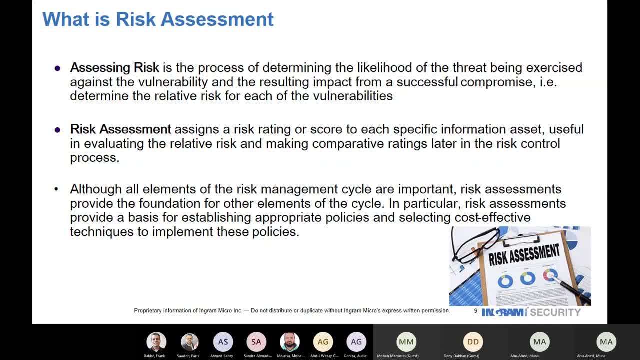 And you classified your assets And then you need to put risk rating And you relate to the likelihood and the impact of each assets Which cause risk, So useful in evaluating the risk, The relative risk, And making comparative relating later In the risk control process. 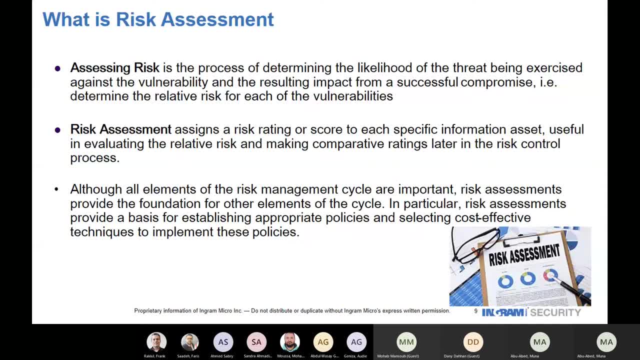 Although all elements of the risk management cycle are important, Risk assessments provide the foundation for other elements of the cycle. In particular, risk assessments provide places for establishing appropriate policies And selecting cost effective technique to implement these policies. That means when you do your table. 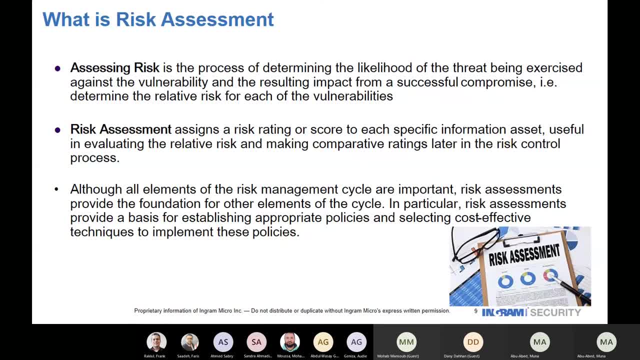 Or your risk register, Let's call it- We'll speak about the risk register later- And you successfully classified everything. You successfully mentioned the likelihood, The, let's say, the impact of each assets, Or to finally classify the risk of your assets. 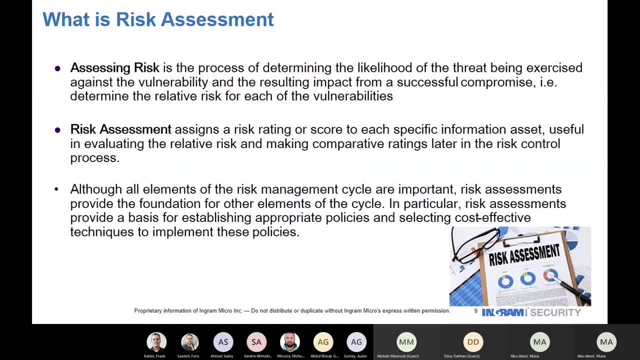 This will end up with establishing a plan, And then you need to find the appropriate way To deal with your risk And to, of course, We are doing all of this process to make it very cost effective For the company To protect or prevent the risk. 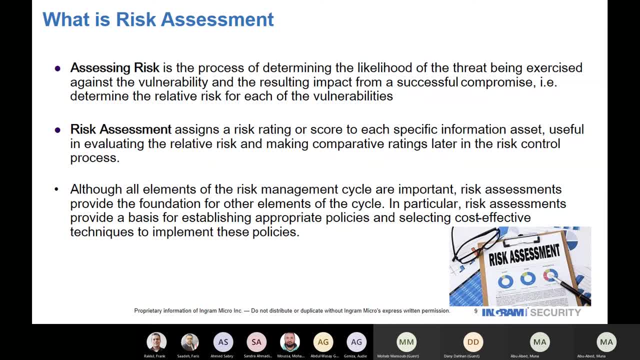 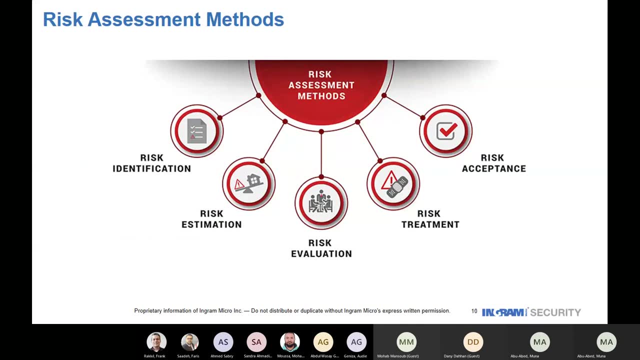 So putting it all in one, In one table We'll find the cost effective technique To implement the policies related to this assets To prevent or, Let's say, To avoid such risk. So what's the risk methods, Assessment methods. 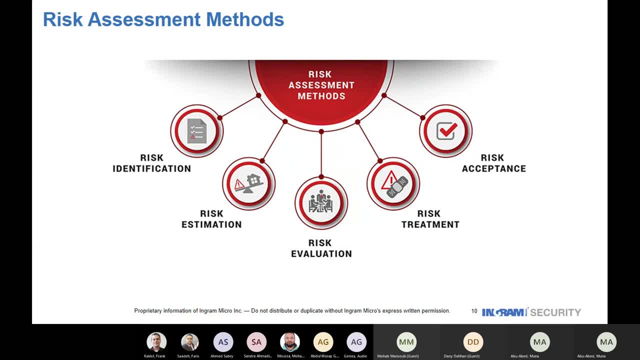 As we said, The first Crucial phase is the risk identification, Then risk estimation, Then we need to do something called risk evaluation And risky treatment And finally risk acceptance, Because whatever the company was trying to always list all the risk. 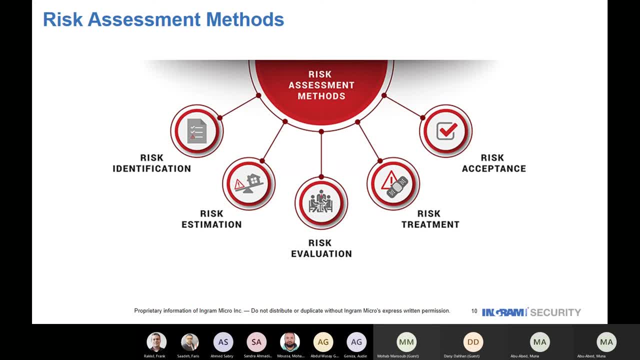 Trying to implement the needed remediation steps, Let's say To close the gaps, To avoid such risk. There is some points And some assets. Let's call it That you cannot avoid the risk, So you need somehow to accept the risk. 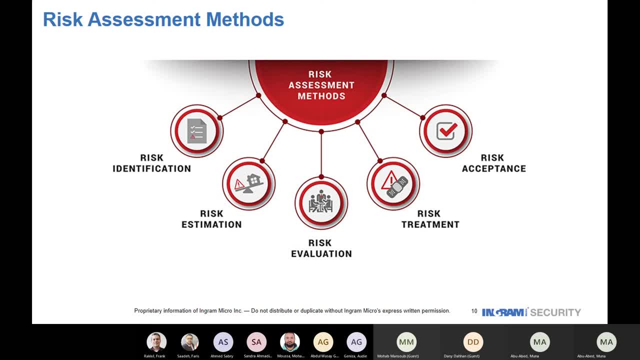 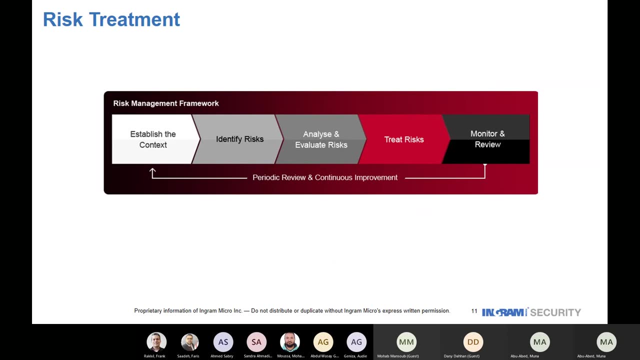 But accept it in a way That's You put all the counter measures Actually To not have any impact to your business. In the risk treatments We establish the context, We identify the risk And we analyze and evaluate the risk. 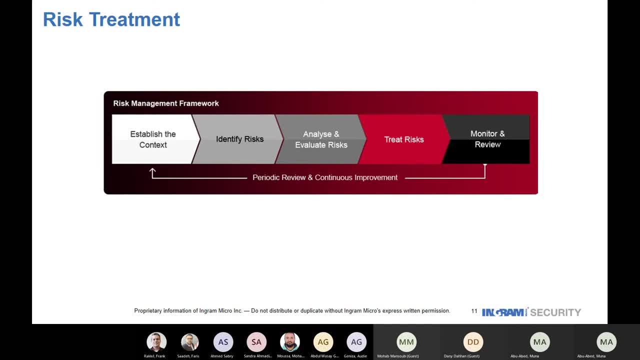 And then we treat the risk And we Monitor and review And this is Like A cycle. So you never stopped monitoring and reviewing the risk And you keep always establishing the context, Because You know cybersecurity is something very dynamic. 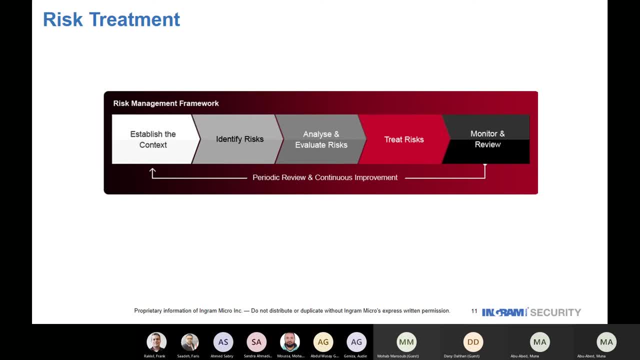 So Just identifying the risk one time Will never help. So you need to keep identifying The risk, You need to Analyzing and evaluating the risk, You need to keep Treating the risk. It's something continuous, So there is some. 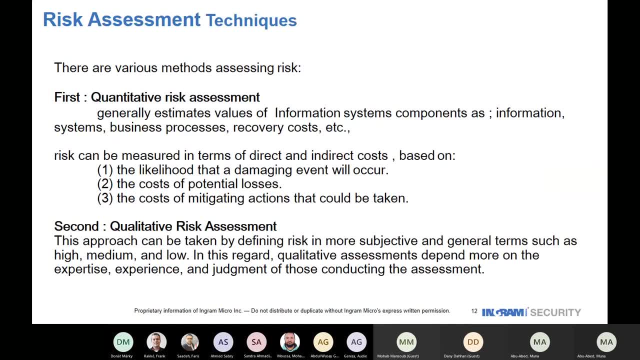 Risk treatments or risk assessment Techniques. So The first technique is Quantitative risk assessments. So In the quantitative Quantitative risk assessment It's Estimates the values of the information systems component, Such as the information systems, The business processes. 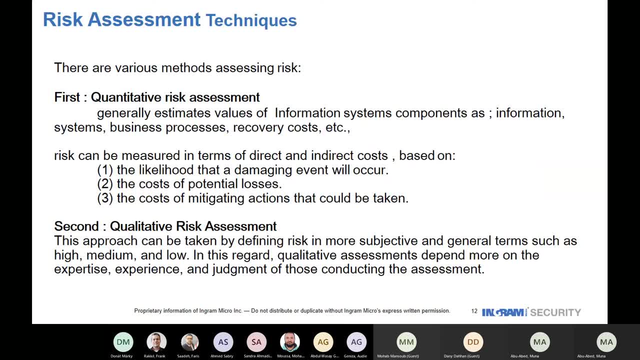 Recovery cost and so on, And the risk can be measured In terms of direct and indirect costs Based on the likelihood That's A damaging events will Cure The cost of potential losses And the cost of mitigation That could be taken. 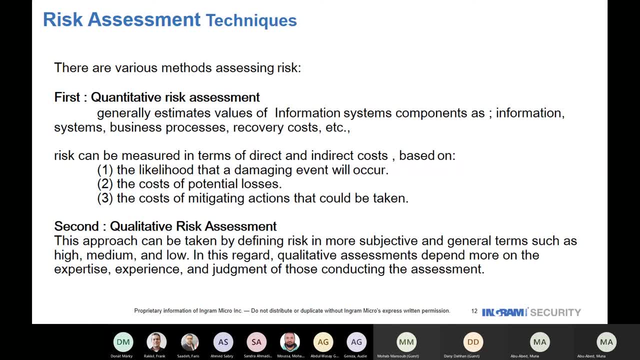 And the second technique Is a qualitative Risk assessment, So this approach can be taken by defining risk In more subjective and general terms, Such as high, medium and low, And I am I'm sure that's the people who Was working on the risk assessment. 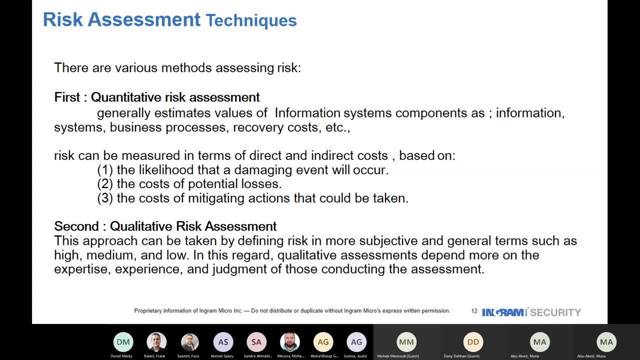 And the risk register And Even the gap analysis. They know What's the qualitative risk assessment, So They always saying this: High, Medium, Low Categorization In their risk register. So, In this regard, The qualitative assessment, 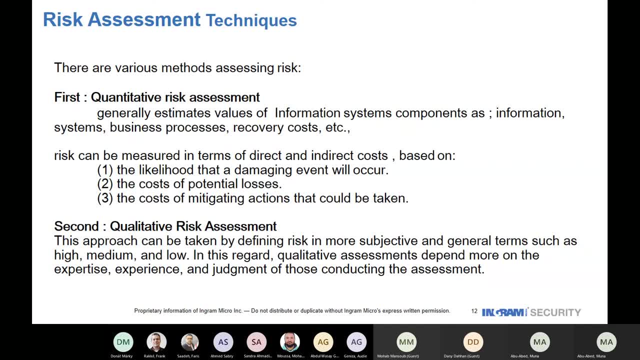 Depends more On the Experts, Experience And judgment Of those conducting The assessment. So If I'm doing the assessment And, As per my experience, I need to define this risk By medium, Then I can Add it. 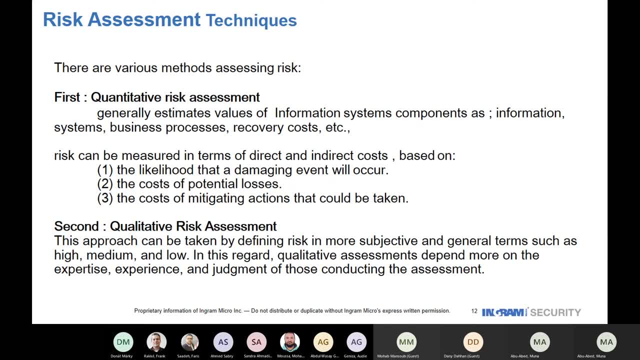 To The Risk register Or Identify this risk As a medium Based on my experience. So The qualitative Is not Relaying On the Cost, It's not Relaying That much On the likelihood. 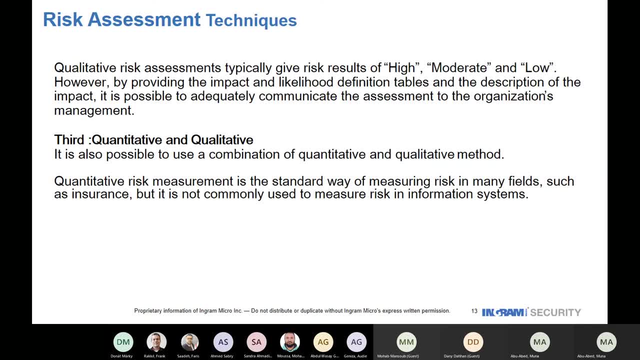 Like The one Which is In the Quite Qualitative Risk assessment. So The qualitative Risk assessment Typically Gives A risk Result And likelihood Definition Table And the description Of the impact. 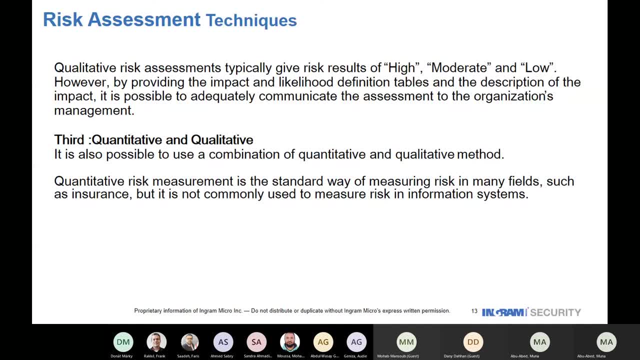 It's very important To communicate The Assessment To the Organization Management. The third One Is Like A combination, Actually, Between Quantitative And Qualitative, So It's Also Possible. 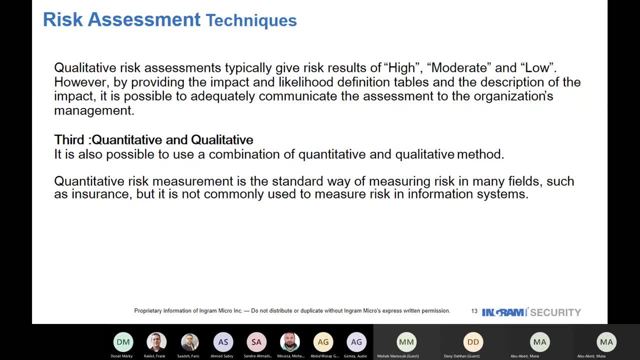 To use A combination Of Risk Assessments Such As Insurance, But It's Not Commonly Used To Major Risk In Information Systems And That's Why Maybe 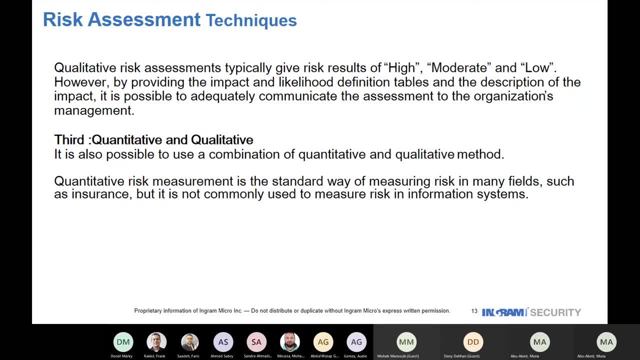 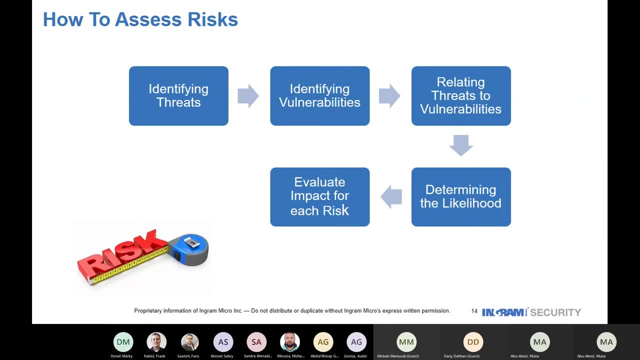 People Who Are Working In The Information Security Or On Risk. So We Spoke About Risk Identification Right, Which Is, We Said, It's Very Crucial. 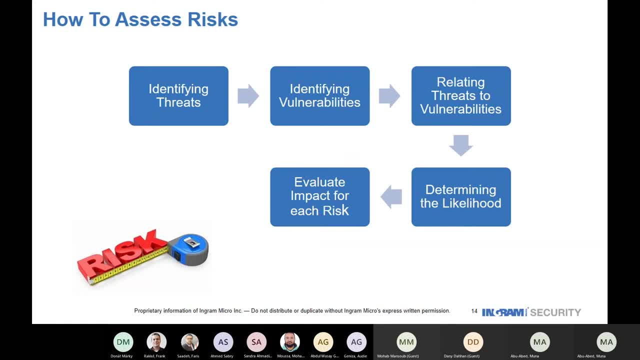 So How We Identify Or How We Assess The Risk. So When We Are Saying, We Identify Your Vulnerabilities And That's Why We Are Running, 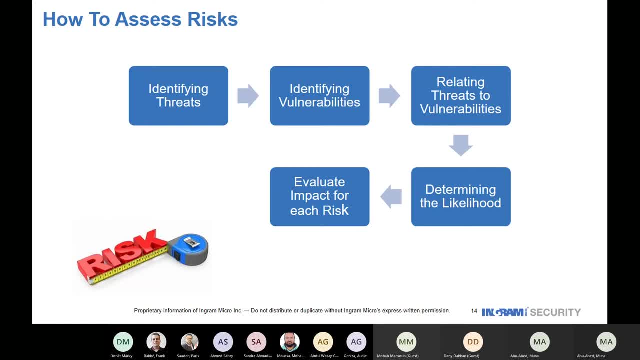 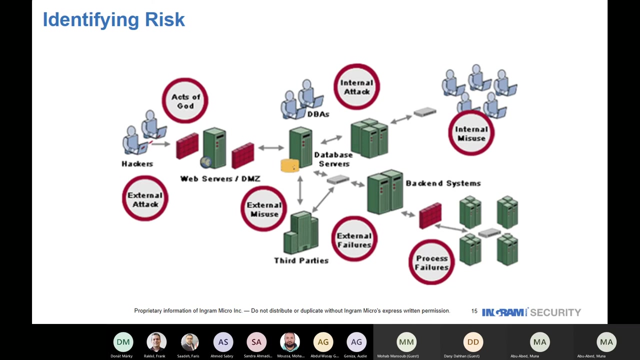 Vulnerability Assessment And Penetration Testing Actually, And Then You Need To Relate The Threads To The Vulnerabilities. So Imagine The Scenario Which I Put. 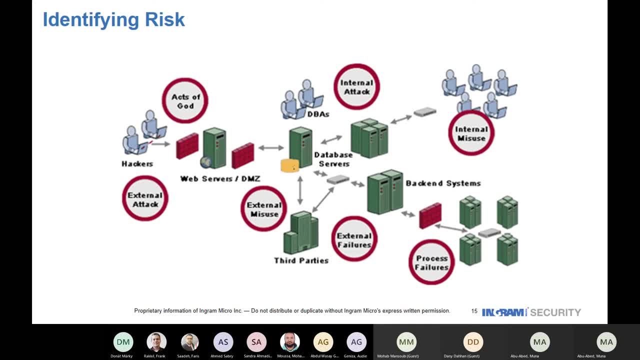 In My Slide Here. So, As You Can See Here In This, Let's Say, Design Of You, Will Start From The External Threads Right And 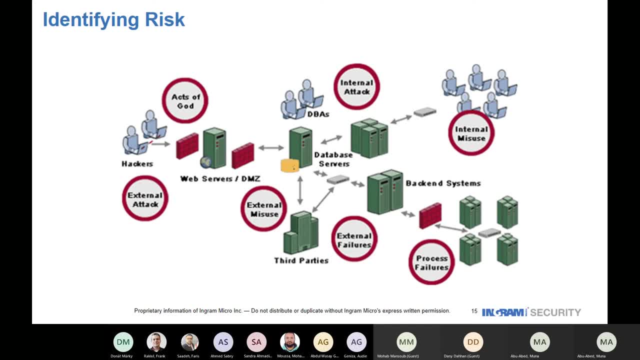 Then We Have In The Middle The Administrators. Let's Say Who Are The DBAs. So We Have Internal Attacks, Right. So We Have External. 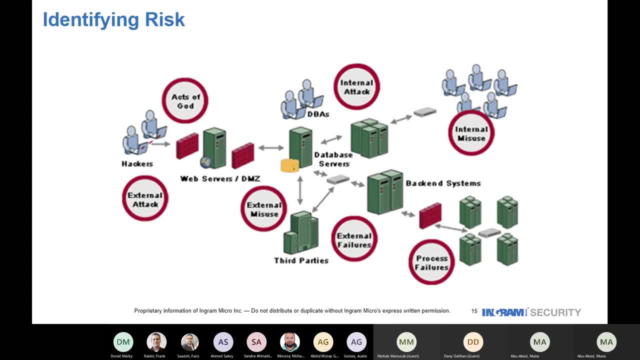 Attacks. Now We Have All The Entities And All The Systems In Their Company, So There Might Be Internal Misuse Right And If There Is, 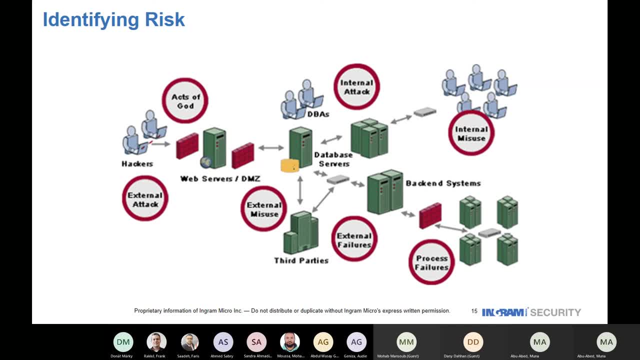 Any Company, Or The Company Is Dealing In Their Back In Systems. So This Is How We Need To Imagine The Factors, Actually The Risk. 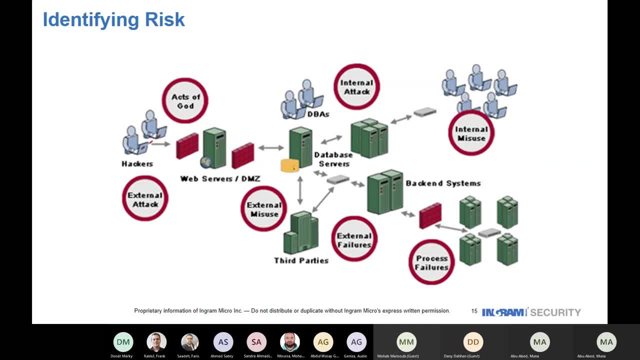 So There Is Also, And Always, Which Is Really Very Crucial For Always, When We Are Doing The Risk Assessment, We Always Make Sure That 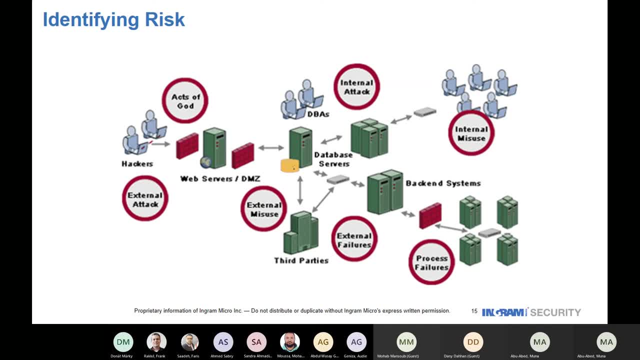 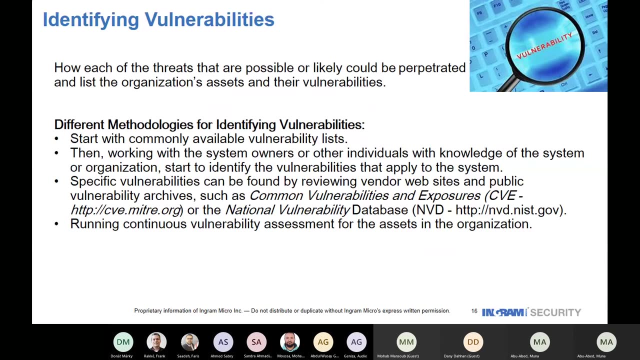 All The Countermeasures, All The Polices Are Procedures Are Applied To Avoid Such Internal Misuse, Because So This Is How We Are Identifying. 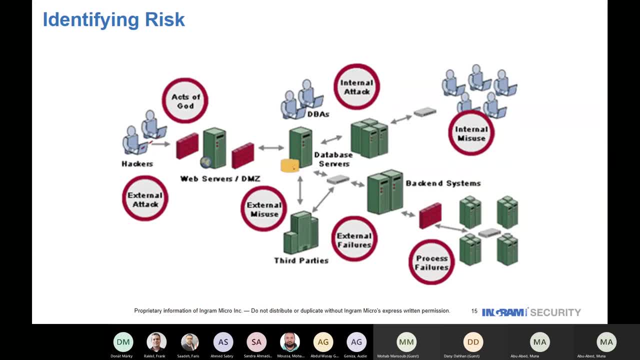 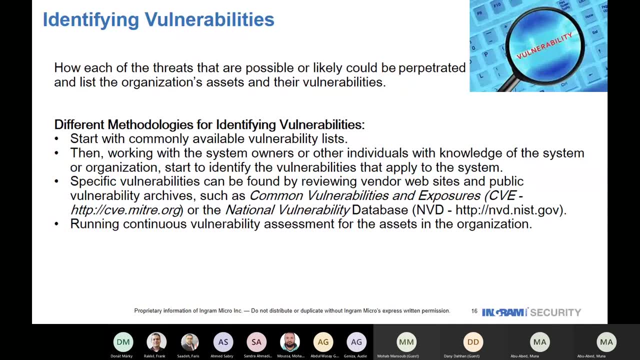 The Threats. All We Need To Imagine That We Are Identifying The Threats Right, Then Identifying The Vulnerabilities. So I'm Sure That There 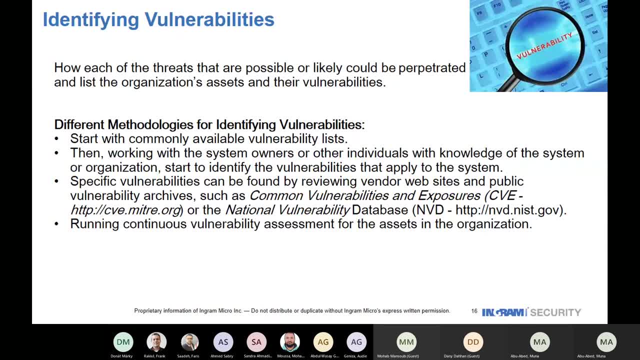 Are So Many Vulnerabilities, Well, What Do We? What Do We Mean Actually? So, And How? Each Of The Threats That Are Possible Or Likely? 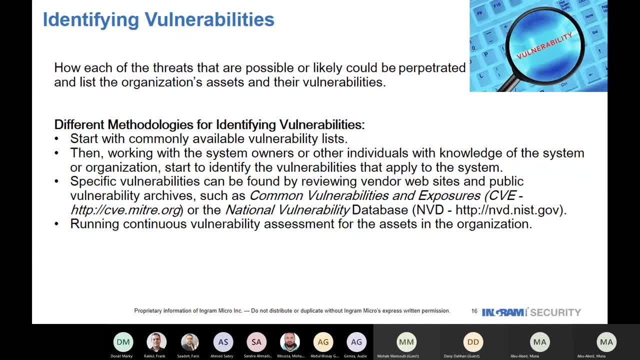 Could Be, Let's Say One Which Is The Most Basic One, Which Is To Start With Commonly Available Vulnerability Lists. So If Some, Some, 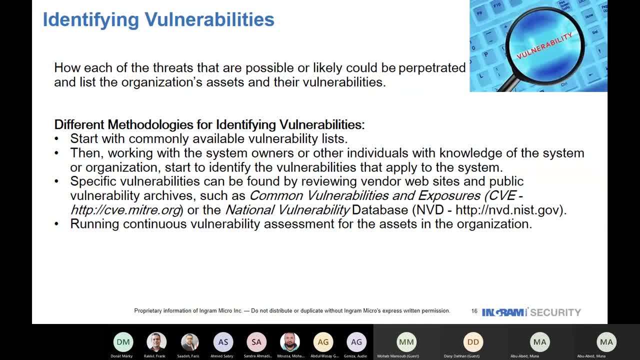 Some Companies. They Still Don't Have This. Let's Say So. All The Admin Needs To Do Is Just To Compare Or To Double Check What. 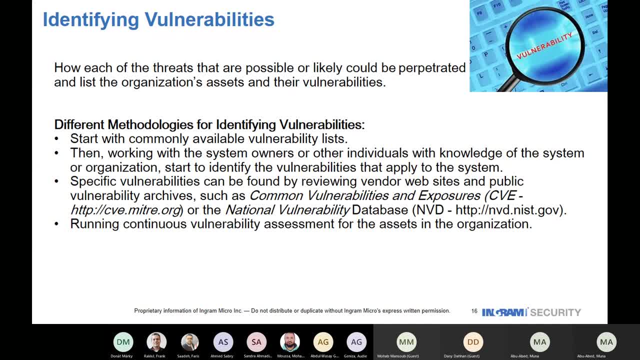 Is The Vulnerability Is Affected. It's On Their Website, By The Way. Affected Because They Will Mention Which Virgin It's Will Be Affected. 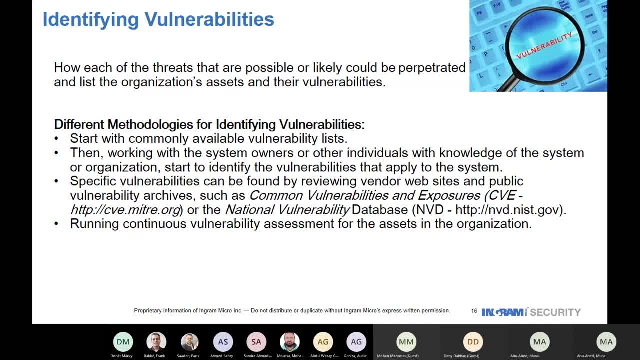 Right. So The First One Is To Start With Commonly Available Vulnerability Lists, Then Working With The System Owners To Double Check For This Cisco. 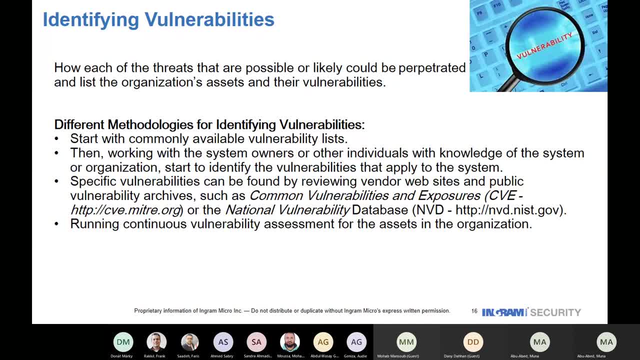 Let's Say Switch Model, To Double Check What's The Vulnerability Affecting This Virgin Or Us Virgin, Of This Switch Or This Router, And 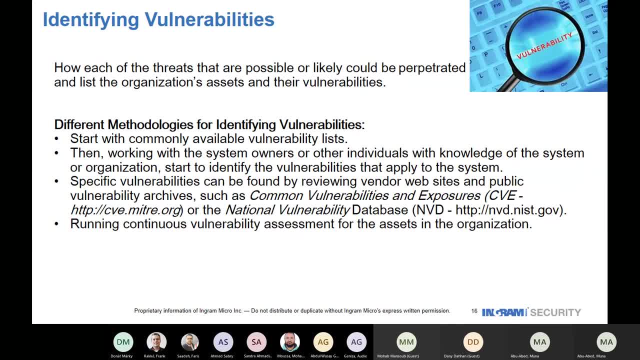 So Specific Vulnerabilities Can Be Found By Reviewing Vendor Website, As I Mentioned, And There Is A Public Vulnerability Archives, Such As Common Vulnerabilities. 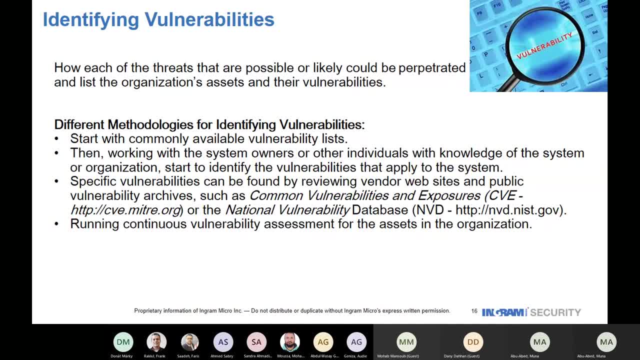 And Exposures It's C B List. Don't Go So. If You Visit To This, This To Website- Actually You Will Find The Recent Websites. 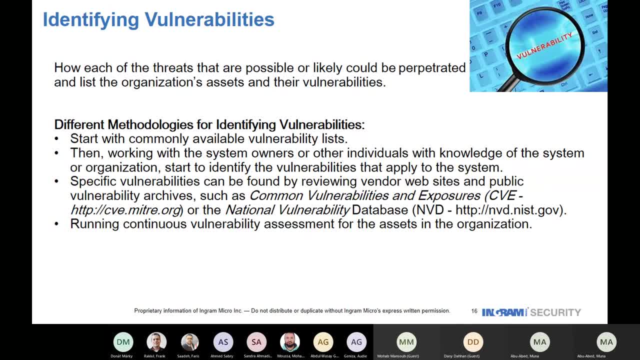 Or Recent Vulnerabilities And Mentioned In That Website And, Most Actually, As A System Administrator Or A System Owner, Or Even The Person Who Is. 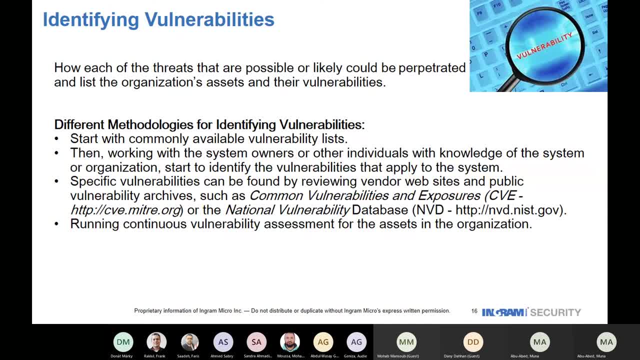 Doing The Risk Assessment To Know Them, Because It's Not Enough. From My Experience, It Requires A Solid Experience And The Operating System As Much. 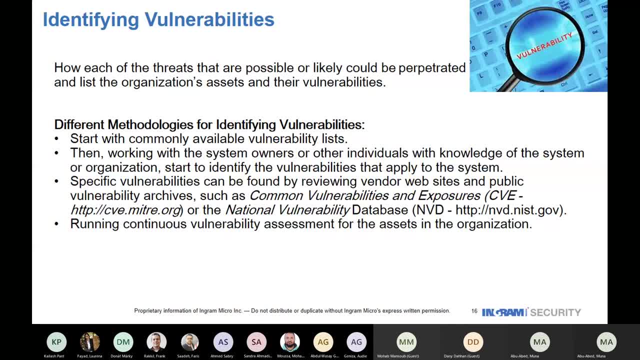 As You Know, Applications And You Dealed With Applications And Operating Systems And Systems. Actually, You Will Be More Familiar With You In The Work. 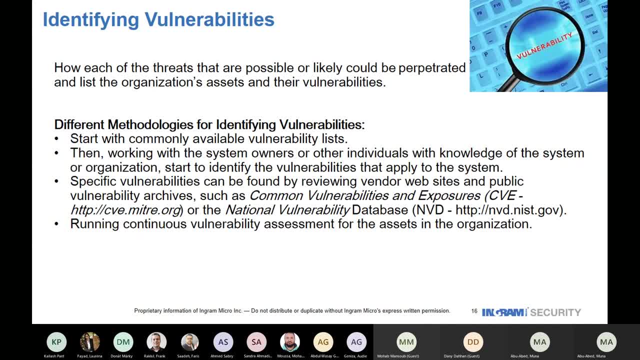 Of Your Employees, And So You Know That You Are Only A Person Who Is Working With You And You Are A Customer, And which is tenable. it's one of the leaders in the market and I personally deal with it. 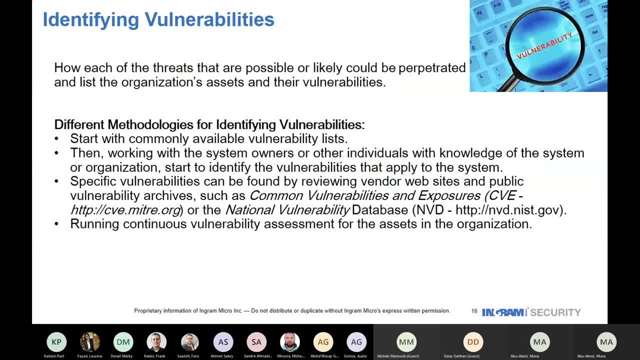 I implement it. it's very easy to deal with it, easy to implement, easy to run the reports, easy to run the vulnerability scan. So I advise any company actually to have this system, to run it internally before having a third party to do the scans for them, Because we know. 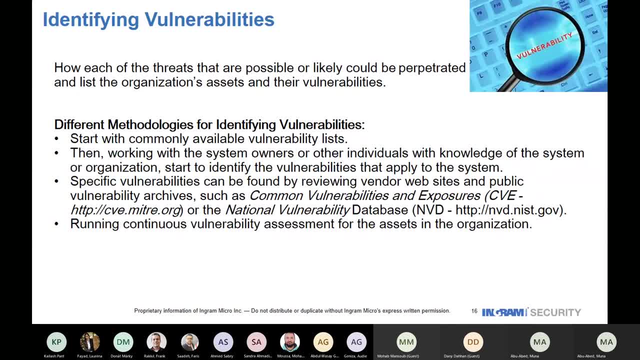 for any security framework implementation you need a third party- even the company is doing the vulnerability management- to do a third party technical assessment services, such as a penetration testing, vulnerability assessment, web application assessment, and to give them a third party report so that maybe the auditor will just compare and find yes. 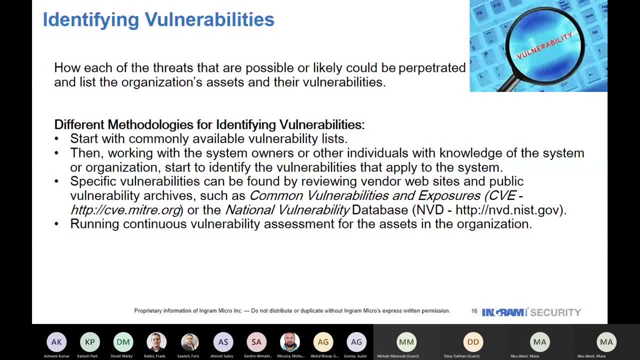 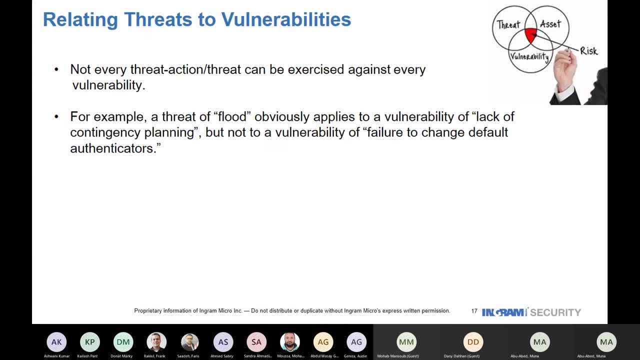 you are closing all the risk or all the vulnerabilities mentioned and so on. And here is a very important step: People, they don't know what's the difference between the threat and the vulnerability. So imagine- and this is a very nice picture actually- so imagine that we have 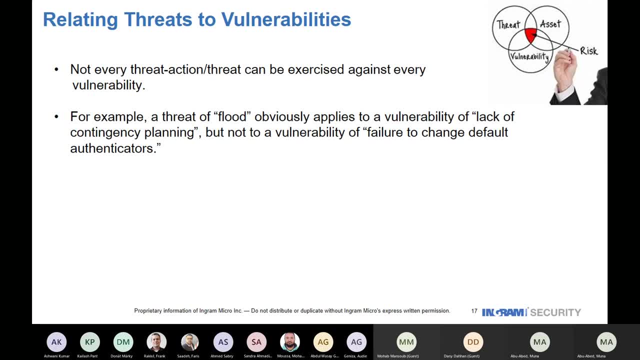 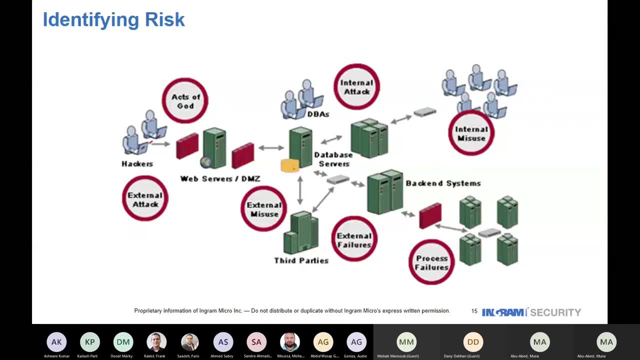 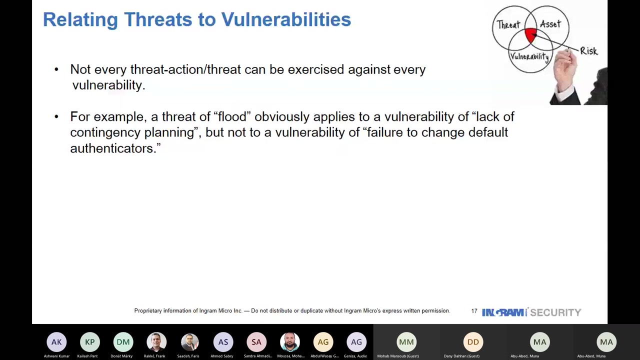 a threat and, as I mentioned, the threat could be, if we go back here, it's maybe coming from hackers, as the system admins themselves and employees, process failures, maybe third parties and so on. So all of this is causing threats actually for the company. 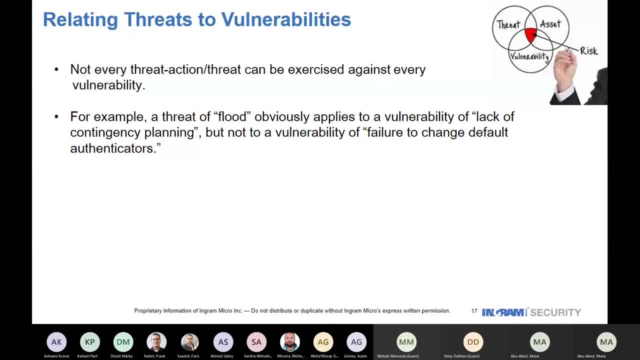 So imagine that we have threats and we have the assets of the company and then we have the vulnerabilities which we discovered. okay, So the risk is coming in between. actually, you know. so not every threat action threat can be exercised against every vulnerability. 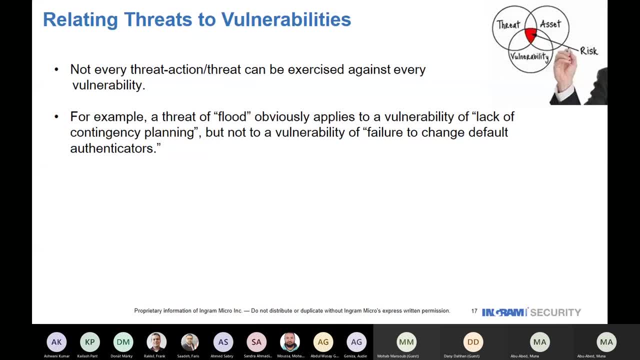 So not every threat is a vulnerability in a simple way. So, for example, a threat of a flood applies to a vulnerability of lack of contingency planning maybe, but not to a vulnerability of failure to change default authenticators, for example. So we need- it's really important for us to understand. 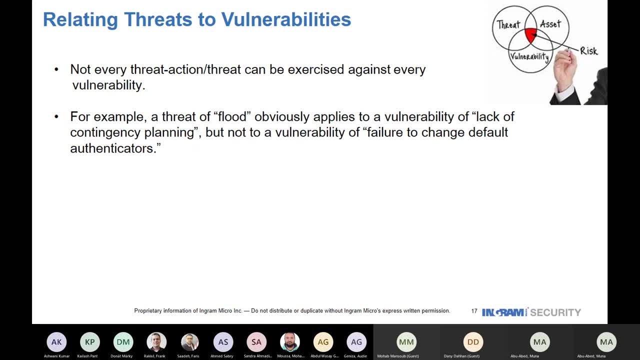 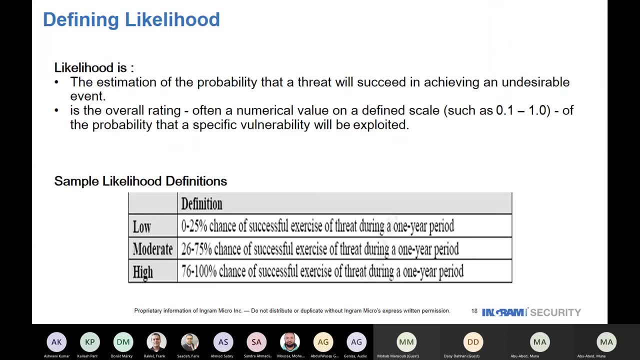 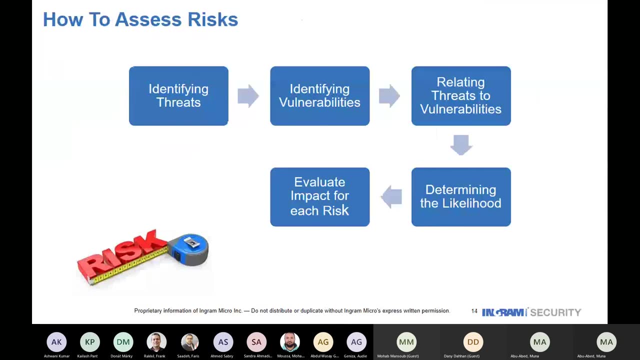 so it's really very important to map the right threats to the right vulnerability, but not always we can map the threats to the vulnerability. And then, well, I mentioned here the steps. so we need to identify the threats, identify the vulnerability, and then we need to match the threats to the vulnerability and it's really very important to determine the likelihood. 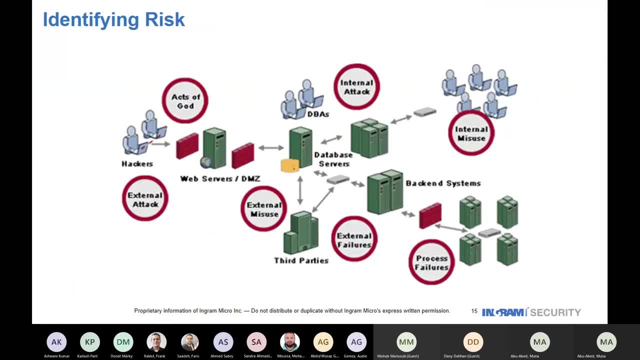 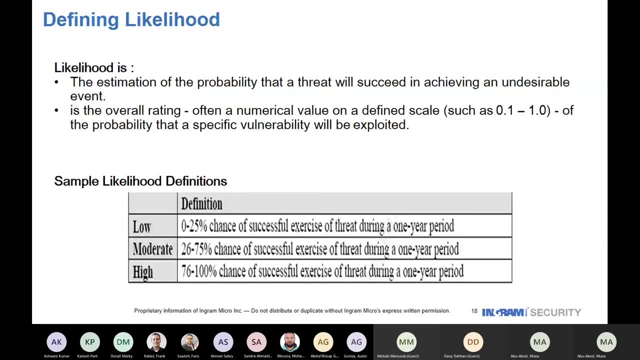 And evaluate impact, each risk. So how we determine the likelihood. So what's the likelihood, The estimation of the probability that a threat will succeed in achieving an undesirable event Is the overall rating, often a numerical value on a defined scale, such as: 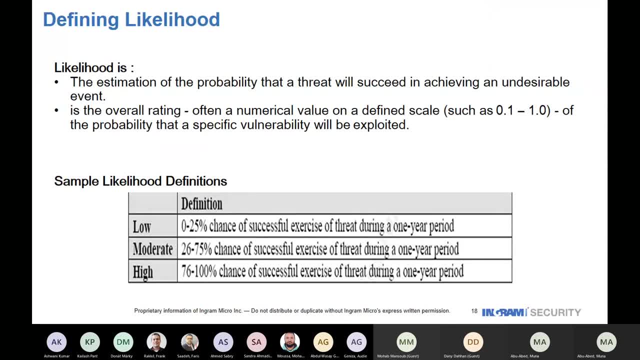 a reduction to one or the probability that a specific vulnerability will be exposed. So, for example, I'll put here a low, moderate and high. So, for example, from zero to 25 percent chance of successful exercise of a threat during a one-year period. 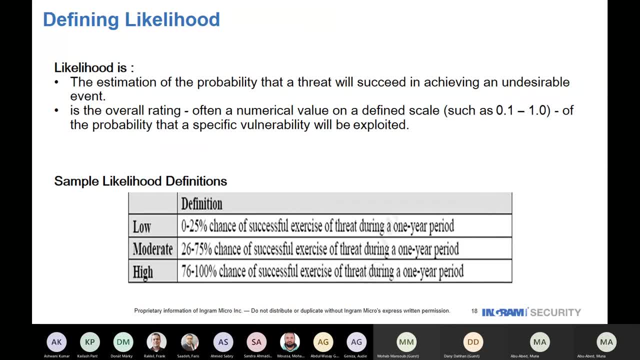 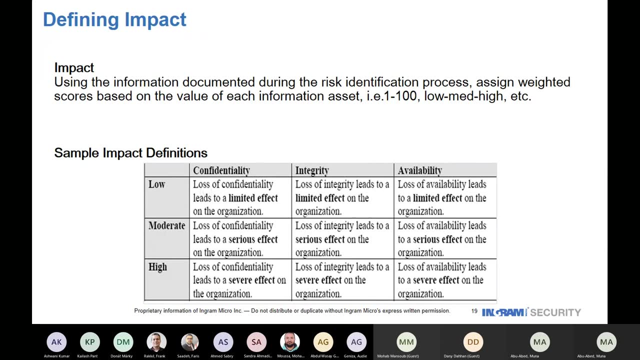 26 to 75,- it's moderate High, from 70 to 75 percent to 100 chance of successful exercise of threads during a one-year period. And then we need to define the impact. So we defined the vulnerabilities, we mapped the 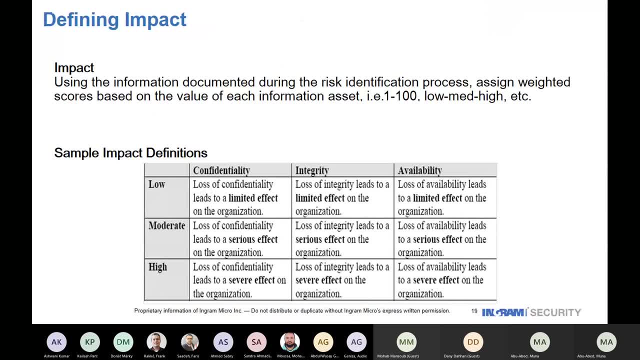 vulnerabilities. we defined the threads and we mapped the threads and the vulnerabilities. we defined the likelihood. Now we need to define the impact. So what's the impact? Using the information documented during the risk identification process, assign weight score based on the value of each information assets. So, for example, from one to 100, high medium. 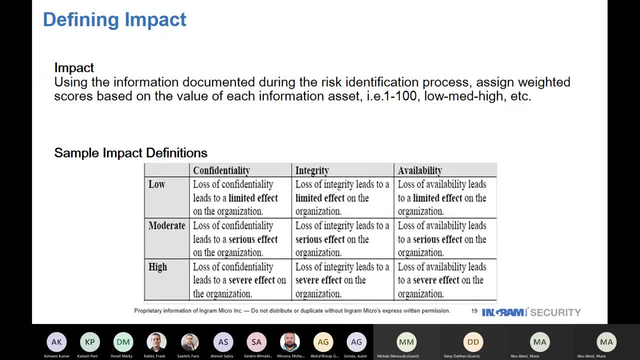 and low and et cetera. So sample impact definition- This is a sample. So, for example, we put low, moderate and high. So I used confidentiality, integrity and availability. So, for example, we put low potentiality, integrity and availability. So, for example, 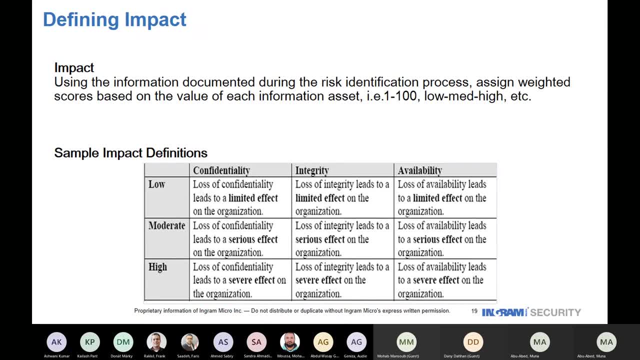 For example, it says I used confidentiality, integrity and availability in terms of the example. this is just an example. okay, so for low loss of confidentiality leads to a limit effect of the organization. this is just an example. integrity: limited effect to the organization. 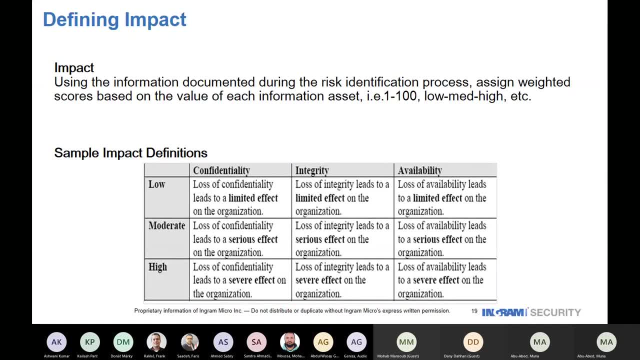 so it's low. if it's serious effects for a confidentiality, i call it moderate. if it's a severe effect, i call it high. maybe someone else will call it critical or crucial. high, medium and low. okay, but you need to define the impact before even starting the risk assessment. 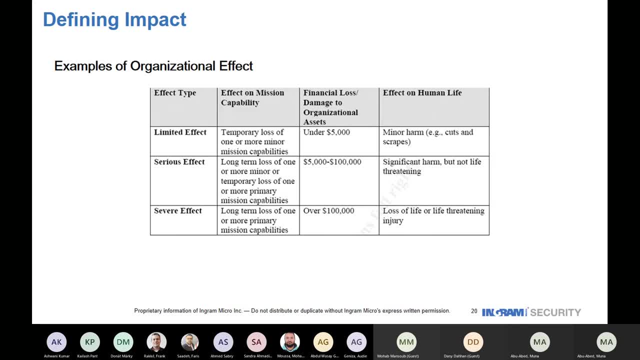 This is another example of organizational effect. so type of effects, limited effects, serious effects, severe effects, risk assessment effect, then effect of mission capability, financial loss or damage to organization assets, effect of a human life, and so on. so this is just an example to show you how we are doing the, the impact or 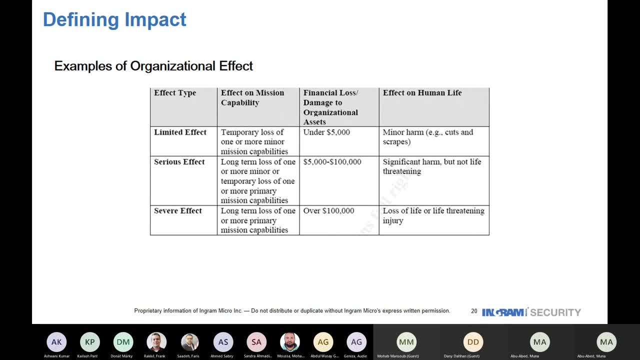 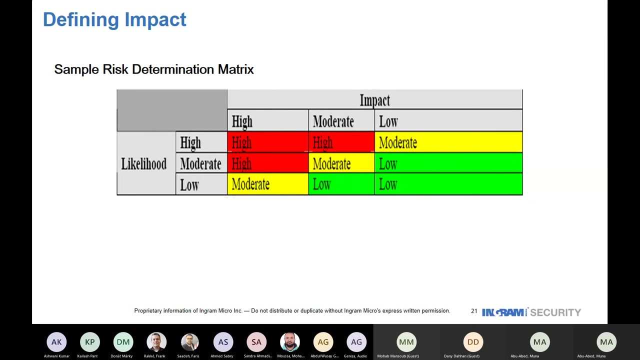 redefine the impact, because it's really very important to have even the impact to the likelihood so that you will have a real, accurate risk assessment document as a final stage of your risk assessment or your management risk management processes that you pass it through. this is the sample risk determination matrix, so you need now to map the likelihood with the impacts. 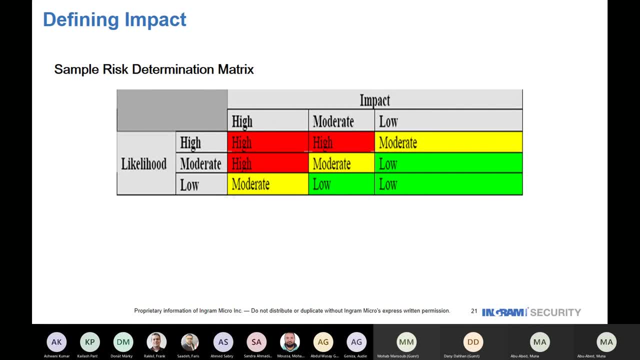 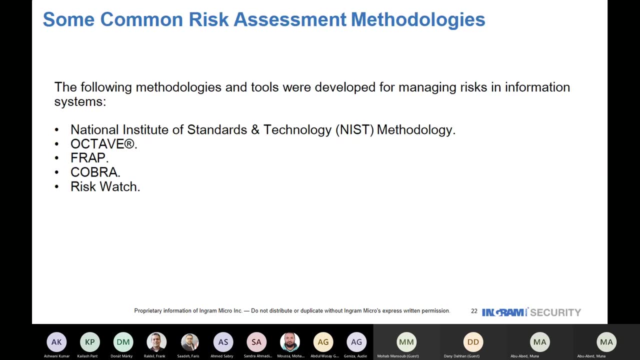 so depends on the category of the risk assessment document. so, for example, high with height will be high, high with low it will be moderate. it depends on what you are assessing exactly. some common risk assessment methodologies. the following methodologies and tools were developed for managing risk in information security. so i i'm sure that you heard about. 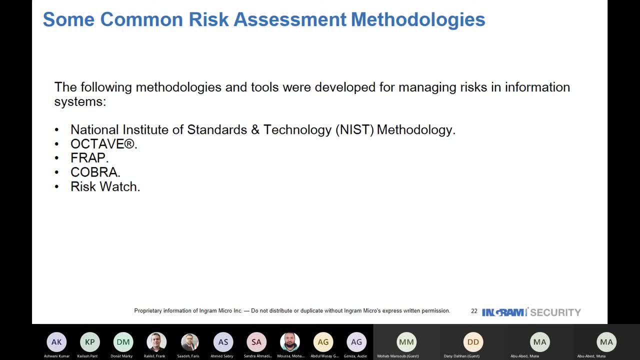 national institute of standards and technologies, which is nest technology, and there is so many other methodologies like risk watch, cobra as well. so people they use different methodologies to run the risk assessment but the most, i mean the most common or familiar methodology here in gcc is the nest or sometime. 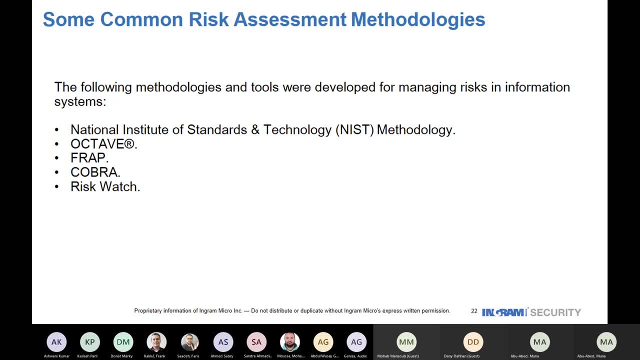 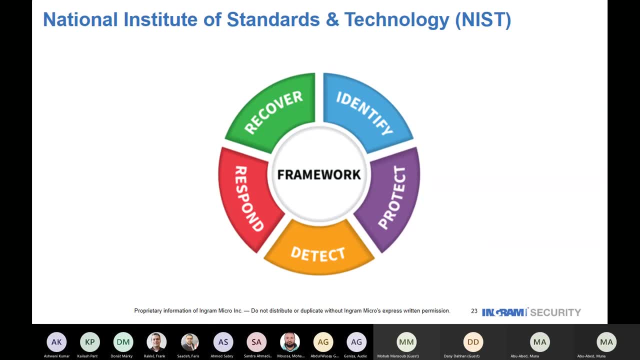 they are following the isr for dubai. so just to give you an overview of the national institute of standard and technology, which is nest, so nest framework. it will have five pillars: identify, protect, detect, respond and recover. and i'm sure that most of you heard about it. 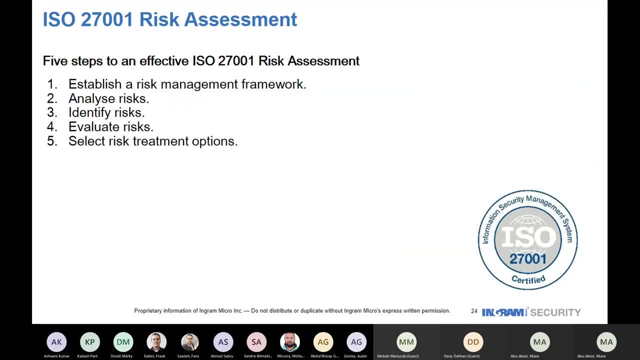 iso 27k based assessment, and here you heard about iso 27k risk assessment also. so there is just an overview of the five steps to an effective iso 27k risk assessment. so the first step is to establish a risk management framework and the second one is to analyze risk, the third one to identify 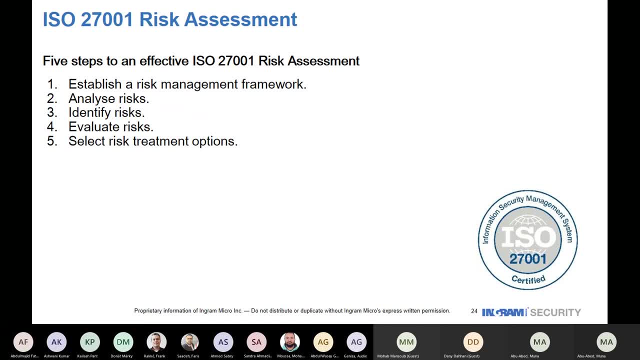 evaluate and select a treatment option. so two points are that. the second is that we have to. So, to be honest, as been my experience working with so many frameworks, the risk assessment, let's say steps, they are almost the same. So the most important is to identify, analyze, evaluate, map the things to each other, which is the threats. 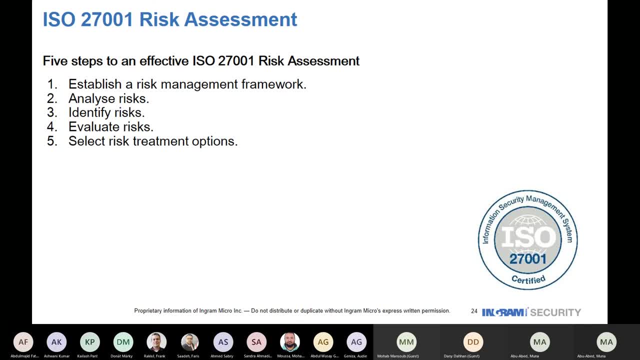 And, as I mentioned, the threats and the vulnerabilities, you identify your way of likelihood and the impact, And then you select the risk treatment options and create your- select or create your- risk Risk treatment plan as well. Now, who's responsible in risk assessment? 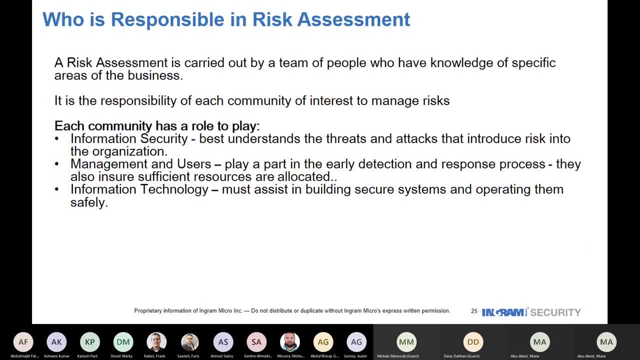 Risk assessment is carried out by a team or people who have knowledge of specific areas of business. It's responsibility of each community of interest to manage risk. Each community has a role to play. So information security, best understanding of threats and attacks that introduce risk into the environment. 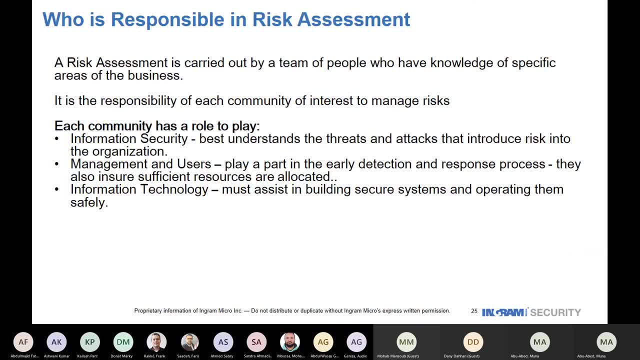 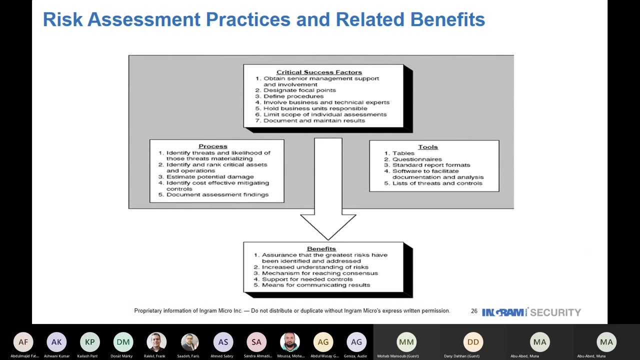 It's the responsibility of the organization. management and users play a part in the early detection and response process. They also ensure sufficient resources are located. Technology, information technology, must assist in building secure systems and operating them safely. And then, what is the risk assessment practices? or what are the risk assessment practices and related? 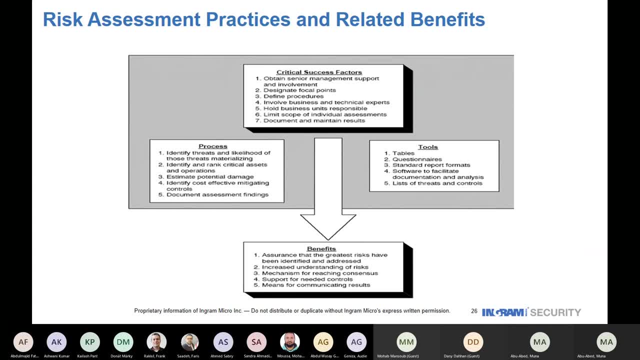 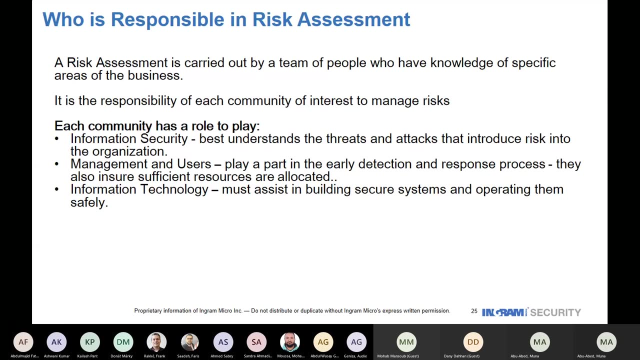 So here I just added this to show you just critical success factors. So it's not enough, to be honest, to get those people included. So maybe just the information security team will work on it and he will have the support from the administrator to give them the needed information. 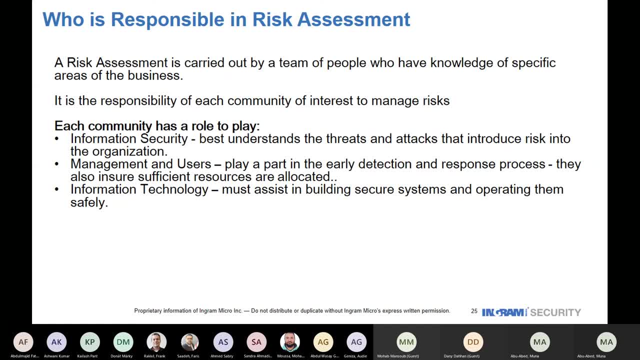 And Maybe from the end users. they will be trained enough to detect and respond, and the IT team they will support them or they will work together to to be responsible on the risk management, let's say plan. But there is a critical success factor: 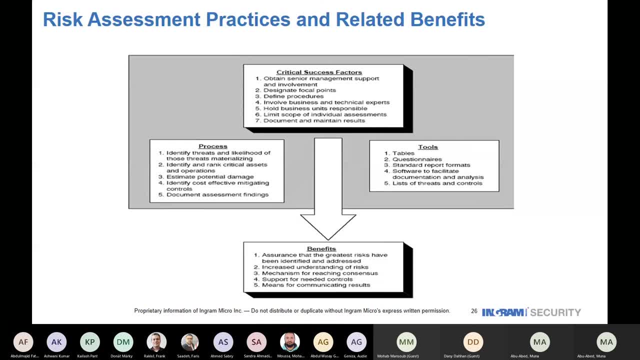 So the first one is to obtain senior management support and involvement, because there is some critical decisions needs to be. So the second one is to obtain senior management support and involvement, because there is some critical decisions needs to be Taken and to be performed as well. 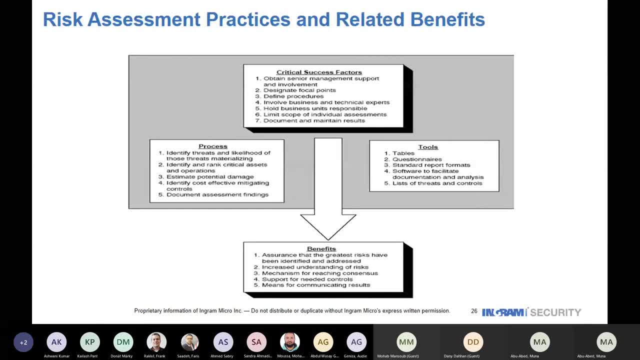 Designate a focal point, define the procedures, involve business and technical expertise, help businesses to be accessible, limit the scope of individual assessments, document and maintain results And then, if it's come to the process, we need to identify the threats, as I mentioned, and likelihood of these threats. 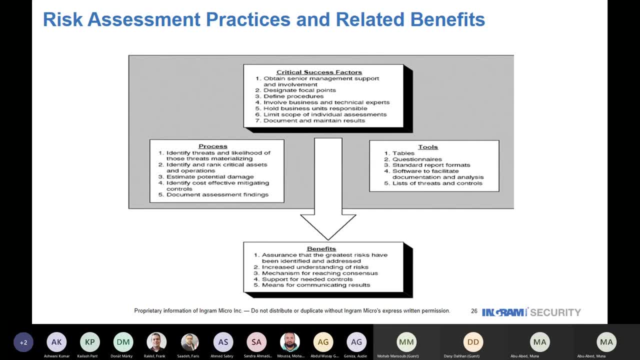 Identify the rank, Identify the risk, assets and operations, estimate potential damages, identify costs, document assessments, findings and so on. So for the tools that will be used, you will tables, questionnaires, standards, reports, formats, softwares to facilitate. 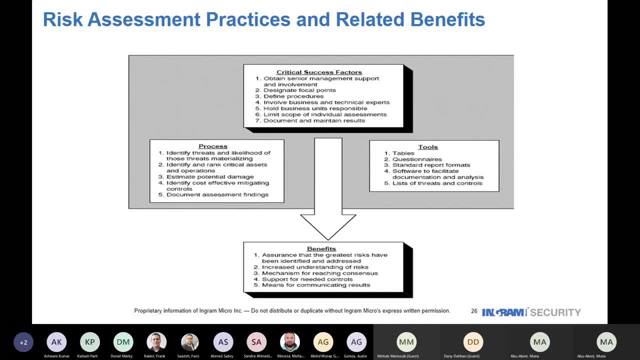 documentations and analysis list of threats and controls. So if we did all this, what are the benefits? Assurance that the greatest risk have been identified and addressed. increased understanding of risk mechanism or for reaching consensus. support for needed controls means for. 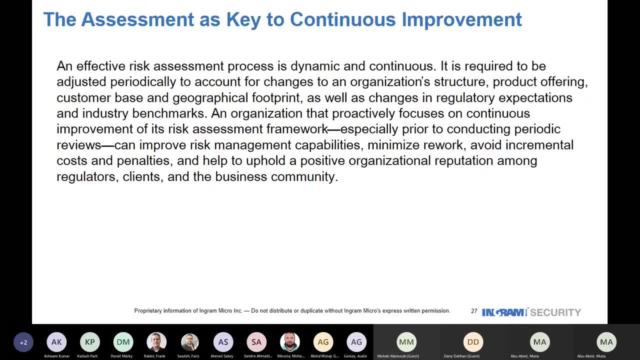 communicating results. And now, what are the benefits? The assessments, which is the risk assessment I mean here as a key to continuous improvements. So an effective assessment processes is a dynamic and continuous, As I mentioned, if the cybersecurity domain is very dynamic, so risk is dynamic. 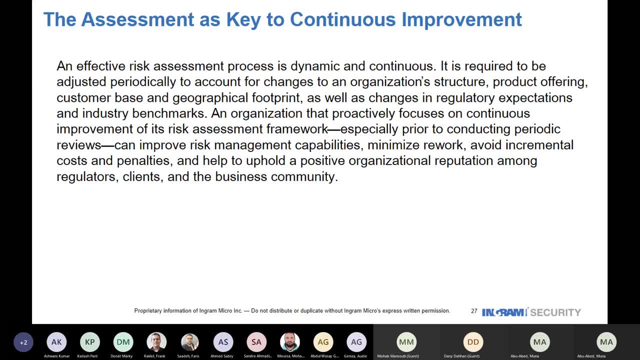 threats never stopped. So the effective risk assessment process. it's also dynamic and continuous. not enough to do it one time and that's it. it's required to be adjusted periodically to account for changes to an organization structure, product offering, customer based geographical footprint, as well as changes in regularity expectations, industry benchmarks and so on. organization that 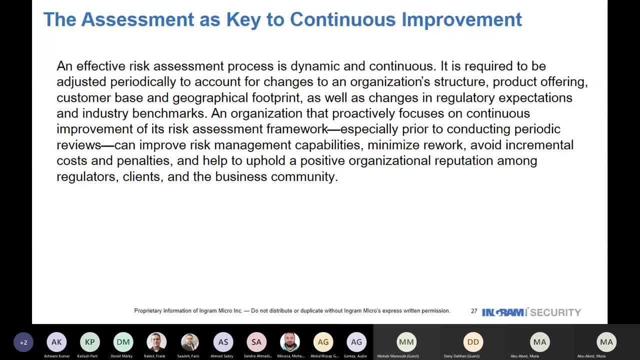 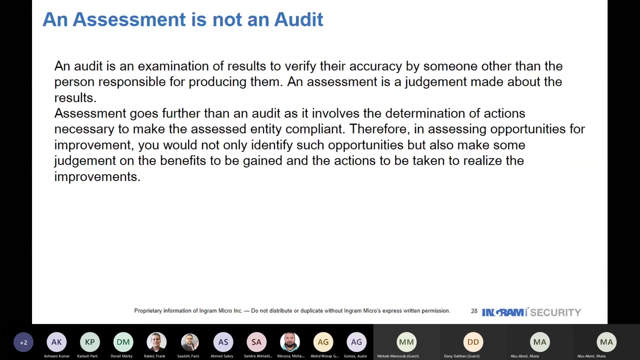 proactively focuses on continuous improvement of its risk assessment framework, especially prior to conducting periodic reviews, can improve risk management capabilities, minimize rework, avoid incremental cost and penalties, and help to uphold a positive organizational reputations among regulators, clients and business community. it's really very important to know that the one who's doing the risk assessment is not an audit. 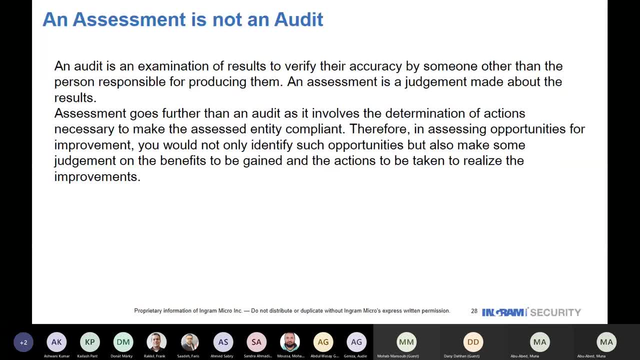 so. an audit is an examination of results to verify their accuracy by someone other than the person responsible for producing them. an assessment is an adjustment made by the results. assessment goes further than an audit, as it involves the determination of action necessary to make the assists entity compliant. therefore, 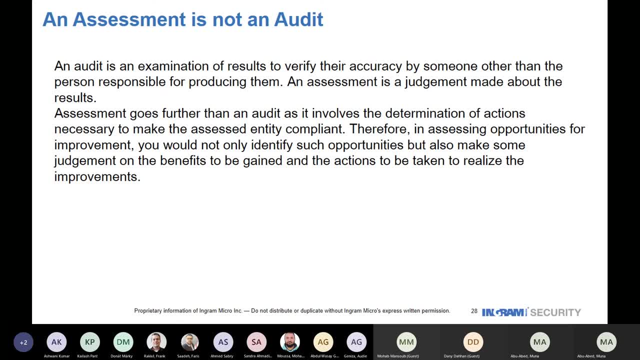 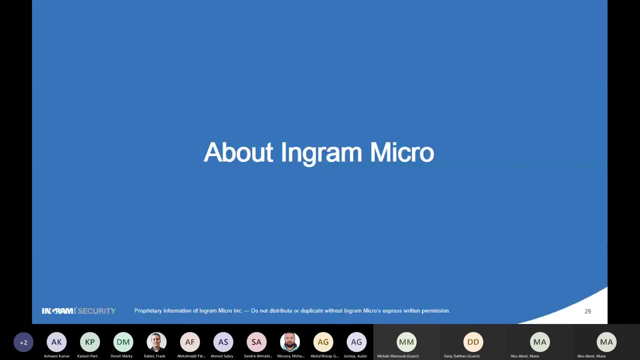 assessing opportunities for improvement. you would not only identify such opportunities but also make some judgment on the benefit to begin and the other actions to be taken to realize the improvements. so this is all about the risk assessment and risk, the risk management and risk identification. for today, i'll just give you a brief about ingram micro. as i mentioned, i'm working in 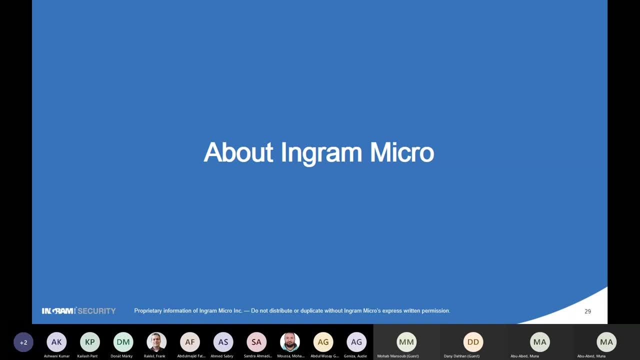 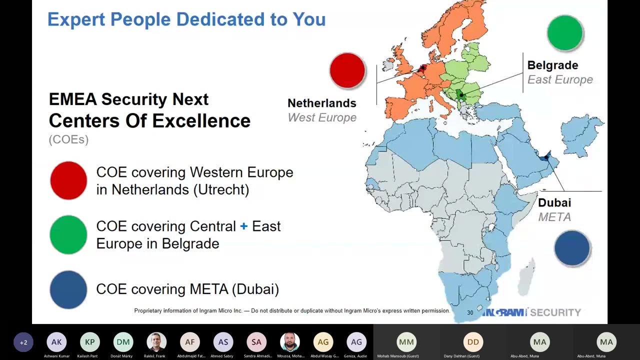 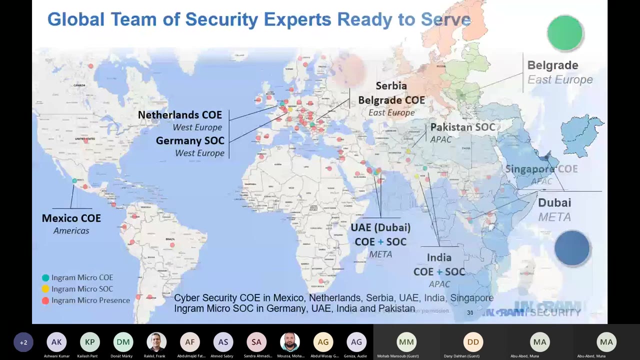 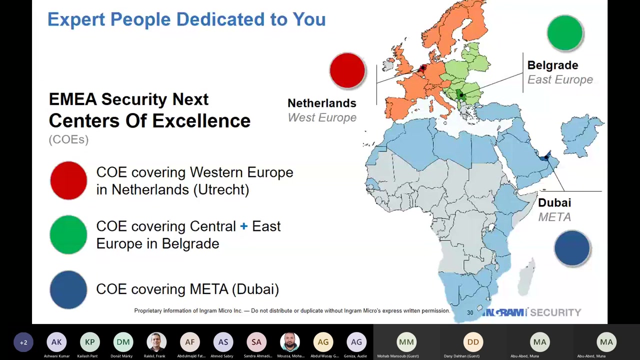 dubai center of excellence, cyber security center of excellence. so um, there is another center of excellence in netherlands and another one in belgrade, in addition to the one which i'm working with in in dubai. so we are trying to cover all uh europe and uh, actually, india countries. 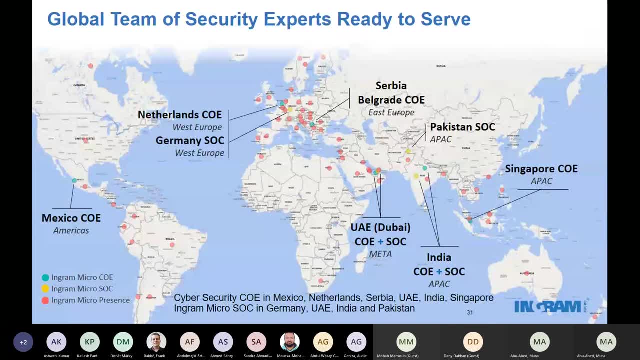 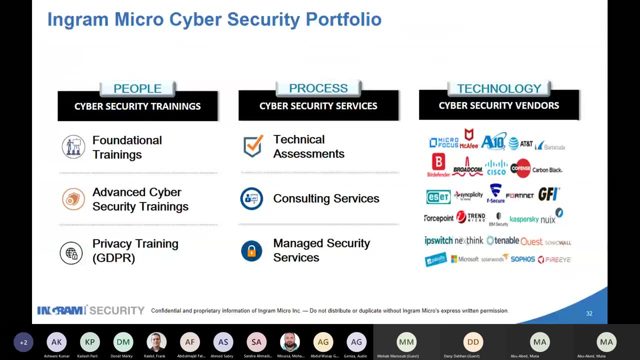 um, in ingram micro we have different. so we have uh in india, so in pakistan, so in dubai and so in germany. and what uh is our portfolio? i'll make it very simple for you. we are trying to cover all pillars, so we are trying to cover people. 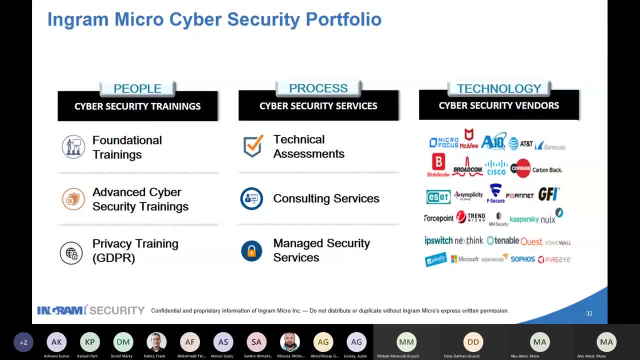 because they are the most important factor of risk. so the people we are doing training for them. so, from fundamental trainings to the most advanced training, in addition to the privacy trainings, and then processes, we are um trying to cover it by having technical assessment services such as vulnerability assessment, penetration testing and so on, consultancy services and 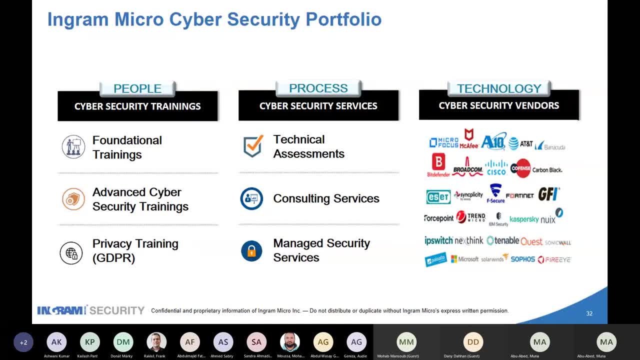 part of it. we do the gap assessment, the gap analysis and the risk assessment and any security framework implementation. and then we have our many security services and, of course, as you know, ingram micro is the biggest distributor uh in the world. so we're a distributor, so we are handling uh more than 27 different cyber security vendors. one of them is 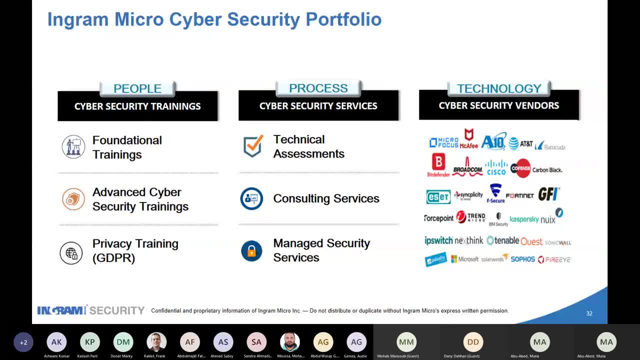 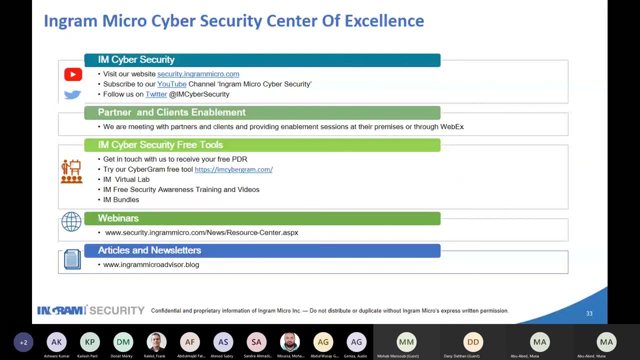 uh a10. we have ibiswitch, we have tenable, we have gfi, we have mcafee, we have cisco, we have sophos and so other um and many other big names in the market. so, um, just give me one minute from your time to speak. our uh free. 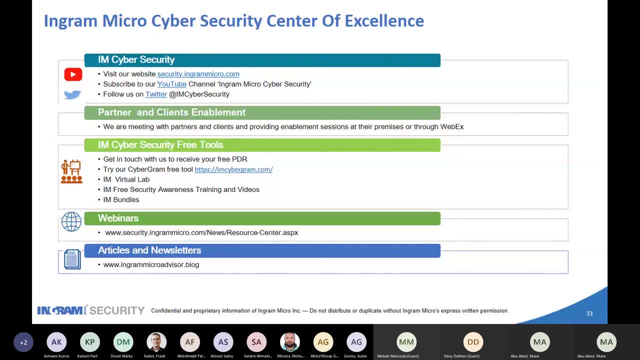 two tools we have um, public discovery scanning, um or public discovery assessment, and all what you need, uh, is to give me your domain name of your company and i will run like information gathering to identify the gaps externally um related to your domain name, and this is free of charge. you will have a report with all the findings which i, um the engineer, can. 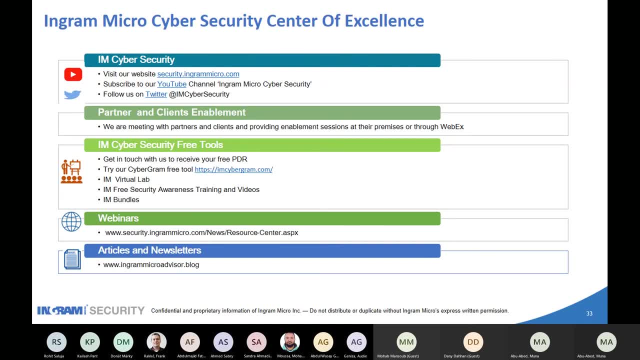 find, and then we have a free tool, which is really a very nice tool. so this is the link for it. it's ingram micro, or i am cyphergramcom, just you need to enter it and you answer some questions and you will have your risk score and the mitigation steps or the remediation steps- how to close the gaps. 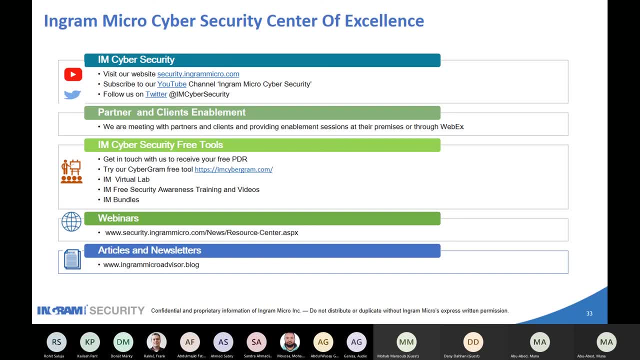 we have a virtual lab, so whatever you need to try as um a product, uh, the engineer for from our site will prepare the lab for you. we'll give you credentials to try the product, to know the features of it and so on. we do a free training and security awareness videos and we have in the micro